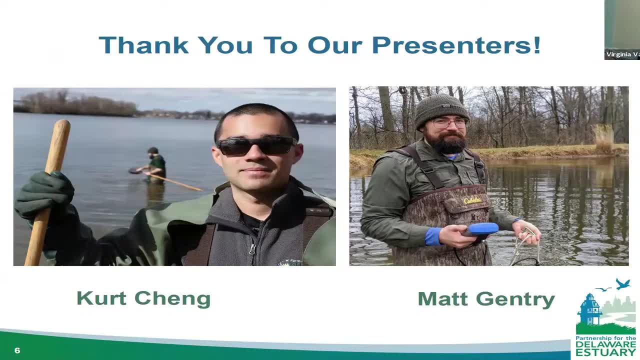 have two speakers, Kurt Chang and Matt Gentry, who will present about freshwater mussels. Kurt will present first, followed by time for Q&A, And Matt will present second, also followed by time for Q&A. So, as a reminder, please use the Q&A function. 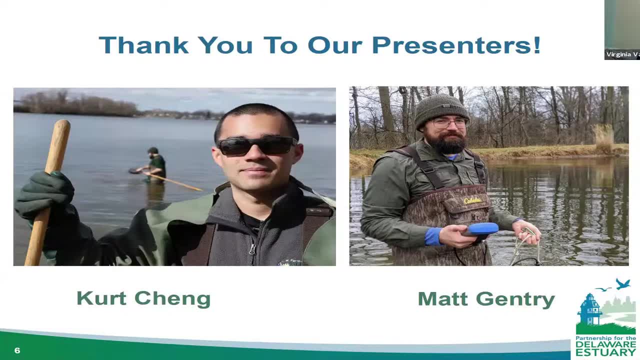 and Emily will be going through that to see if there's any common questions that arise and we can filter those in. after the presentations And, real quick, I'll introduce both of our speakers, And so Kurt and Matt, when I'm introducing you. if you can turn on your video just so folks can see you. First we have Kurt Chang, who is the Director of the Department of Water Resources and Natural Resources at the University of Delaware. First we have Kurt Chang, who is the Director of the Department of Natural Resources and Natural Resources at the University of Delaware. 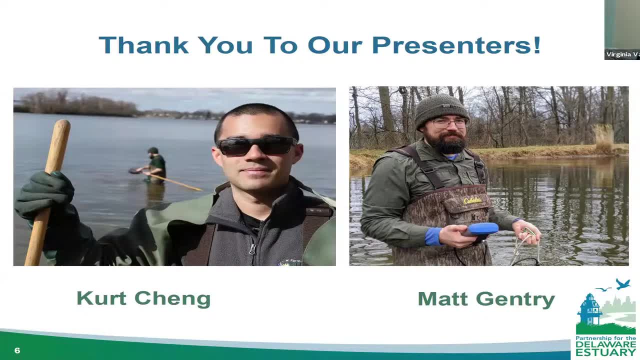 First we have Kurt Chang, who is the Director of the Department of Water Resources and Natural Resources at the University of Delaware. He is the Shellfish Coordinator at PDE. His responsibility is to research the natural benefits provided by various bivalve shellfish found in the Delaware River Basin. 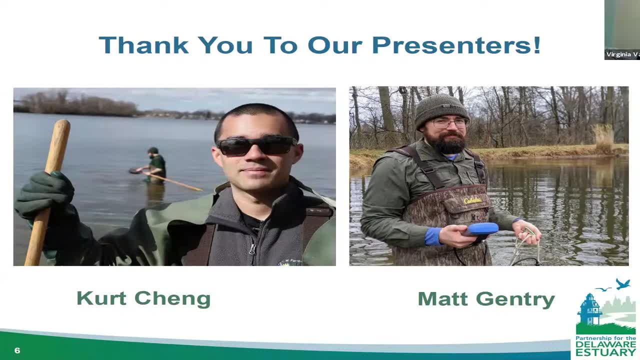 He also helps to advance the freshwater mussel recovery program, which aims to conserve and restore freshwater mussels throughout the region. And our second presenter for the day is Matt Gentry, who is the PDE Shellfish Specialist. And our second presenter for the day is Matt Gentry, who is the PDE Shellfish Specialist. 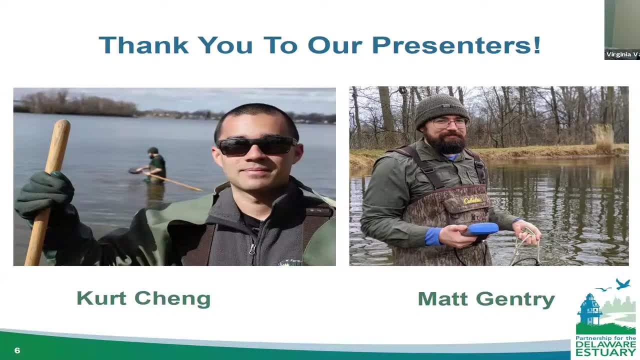 That's always a hard one to say. His work is focused on the propagation and restoration of bivalve shellfish and the evaluation of ecosystem services. He supports freshwater mussel research through innovation and development of novel instrumentation in the field and lab. So with that we can go ahead and get started with our first presenter, Kurt. 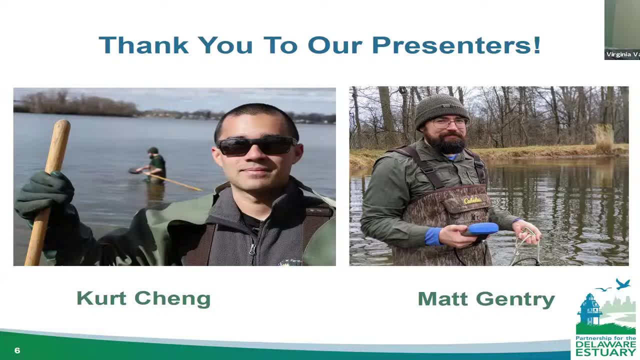 So, Kurt, I'm going to stop sharing my screen and you can go ahead and share yours. So, Kurt, I'm going to stop sharing my screen and you can go ahead and share yours. So, Kurt, I'm going to stop sharing my screen and you can go ahead and share yours. 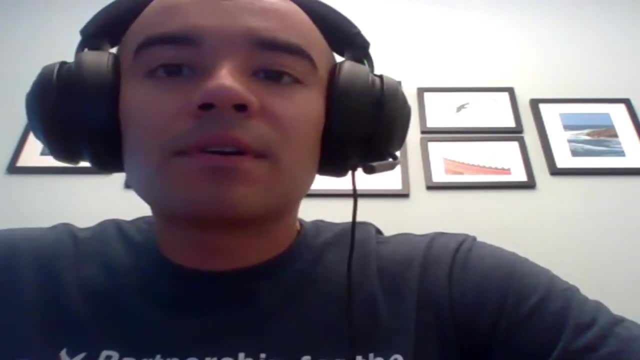 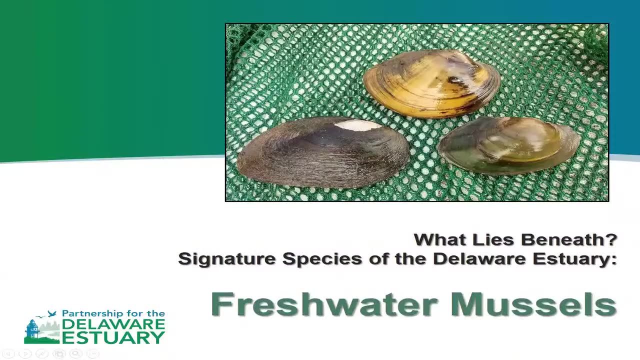 All right. So thanks everyone for tuning in. today We're going to share the presentation here, And so hopefully everyone can see this. So again, yeah, thanks for your interest in freshwater mussels. Let's just go ahead and get started. 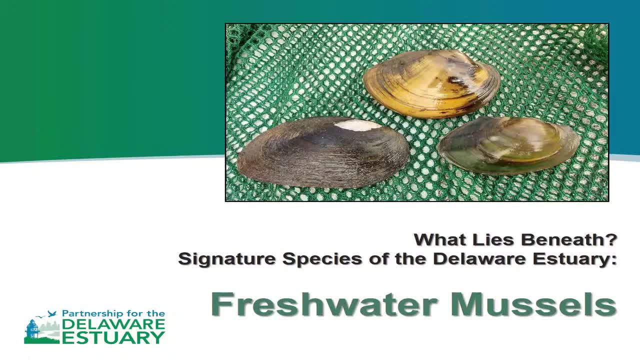 And I just wanted to mention at the beginning that I also have a couple of poll questions to kind of keep people engaged and keep them thinking about what we're talking about, And Matt also has a couple of questions. So stay on your toes. Here we go. 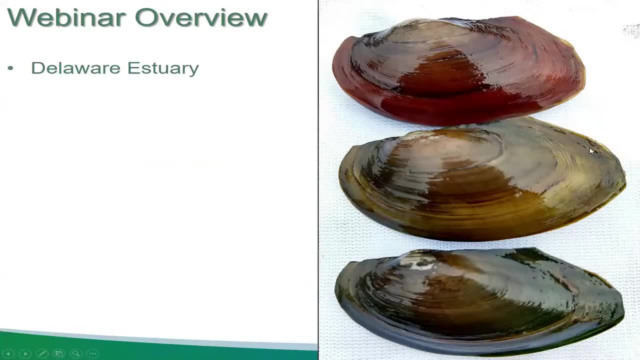 So for this webinar, briefly, we're going to go over just the Delaware estuary. Hopefully, people are generally familiar- We're mostly from the area- but we'll talk a little bit about how the water flows and why that's important for the animals that live in the estuary. 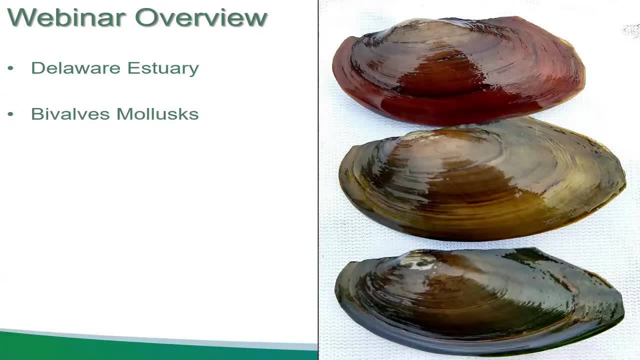 And then we'll talk about bivalve mollusks in general And all kinds of different species, Some that we know, some that we might not, And then narrow down specifically the freshwater mussels, And so that'll be my presentation. 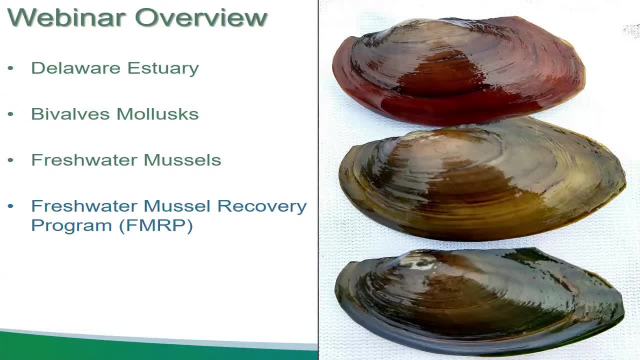 I'll talk a little bit about their ecology and biology, why we care about them, why they're cool, And then Matt's going to talk a little bit more about our freshwater mussel recovery program, as well as the Mussels for Clean Water initiative. 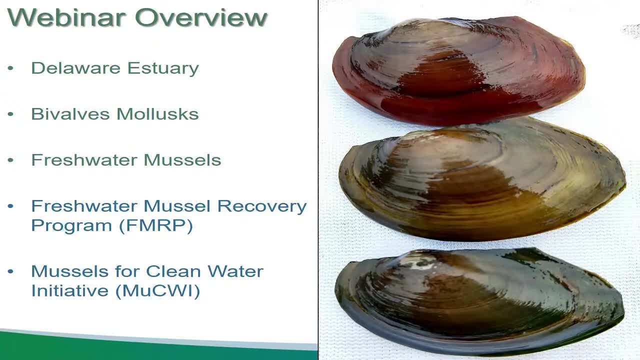 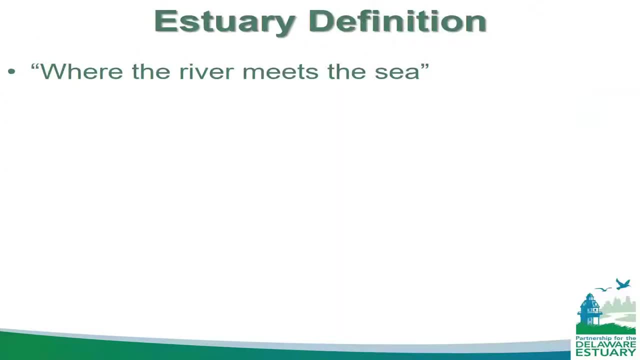 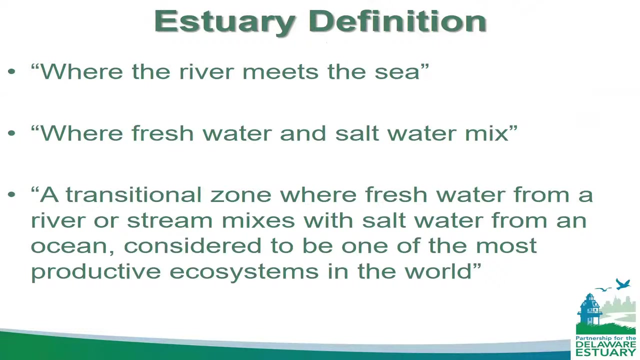 So some of the actual programs that we're putting on at PDE to research, restore and recover freshwater mussels, And then we'll talk a little bit more about the Québec has three Educational ahead: substrate, Cl, 해� 했어. 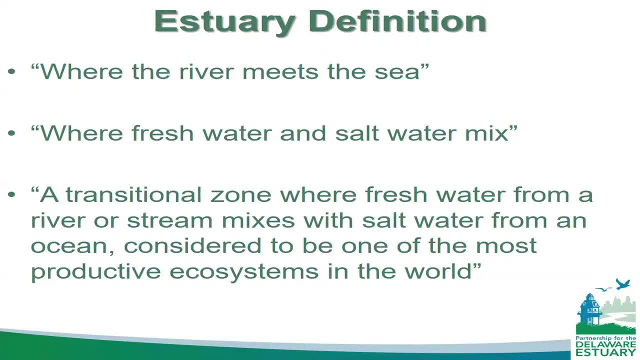 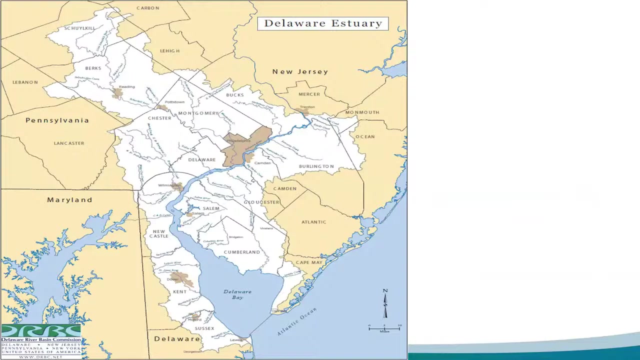 Under the Florida Ontario asto- 搭 Steel, Dr Müller, Sustainable water in the Delaware estuary. as Virginia said before, we have New Jersey on the right-hand side and I think you guys can see my cursors, so I'm just gonna do one of these guys. 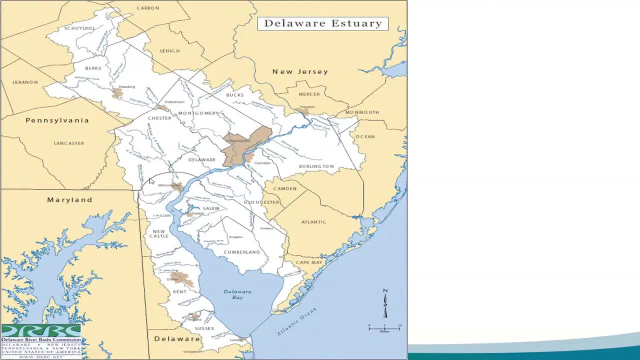 We have New Jersey here, we have Pennsylvania over here, we have Delaware down here, and so you have the Delaware River flowing down and you have the Delaware Bay and, of course, you have the Atlantic Ocean here. So basically you have one-way flow of fresh water. 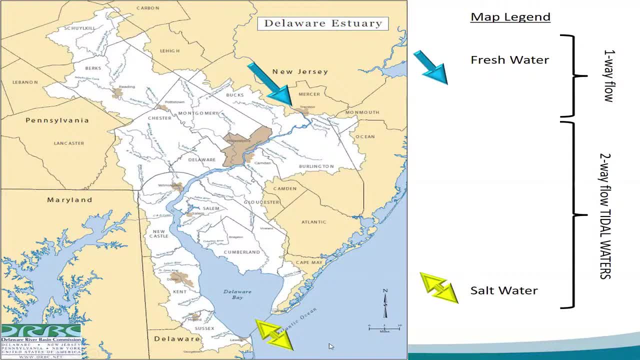 but then you have two-way flow, so that's tidal water of salt water, and so you have the Atlantic Ocean pushing inside the bay and then pushing back out twice a day, And so what this causes is a tide that goes all the way up to pretty much Trenton, New Jersey. 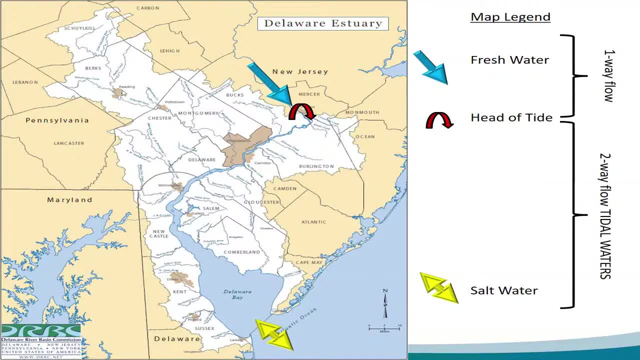 And so Trenton, New Jersey, is considered the head of tide, and what that means is that this fresh water up here only flows one way, until Trenton. This water goes all the way up to Trenton and then flushes back down. 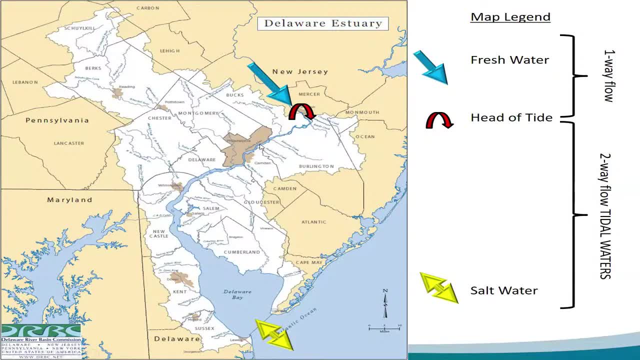 And that's important because that changes the dynamic of the environment in which all these animals live- Fish, birds, bivalves, you name it- And so here we have fresh water all throughout this region generally, and that's different than this fresh water here. 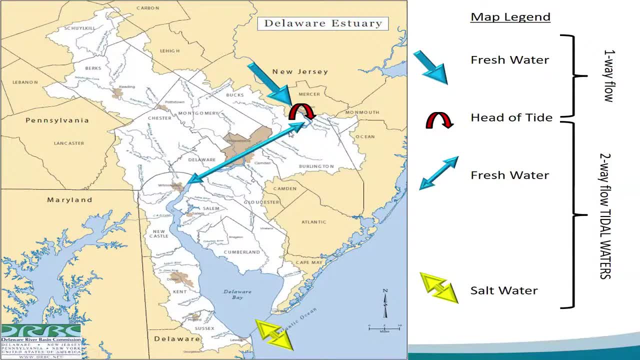 because it's tidal, And so the tide rises and falls in some places up to like six or seven feet, so we're not talking about maybe a foot. It's a drastic change. In addition, because you have this fresh water and the salt water mixing. 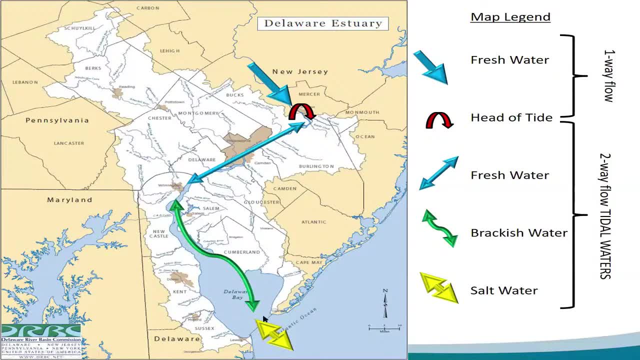 you get this brackish water right in between and there's a gradient, So down here obviously it's a lot more salty than up here, but there's still salt, So no fresh water organisms would be able to live here. 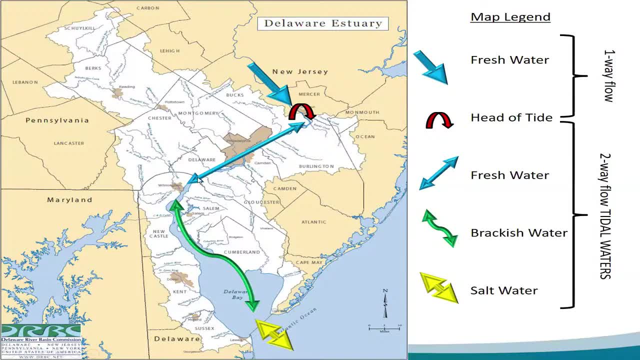 And this is the same for all the tributaries as well. So you have tributaries up here, like the Schuylkill River is completely fresh all the way up to the headwaters, But then down here some of these rivers- 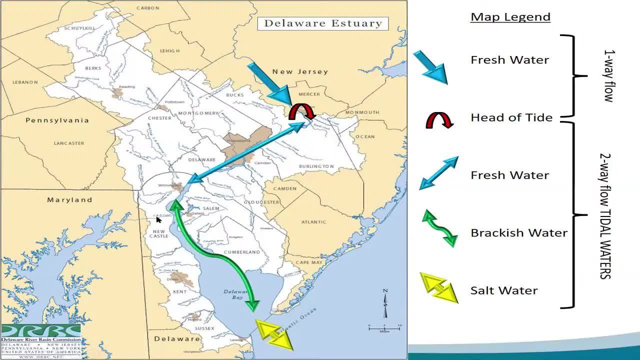 are salty at the mouths, but as you go upstream they become fresh, And so this kind of fresh water, brackish water, tidal to non-tidal flow- resonates throughout the whole estuary And it helps kind of set up all these different locations. 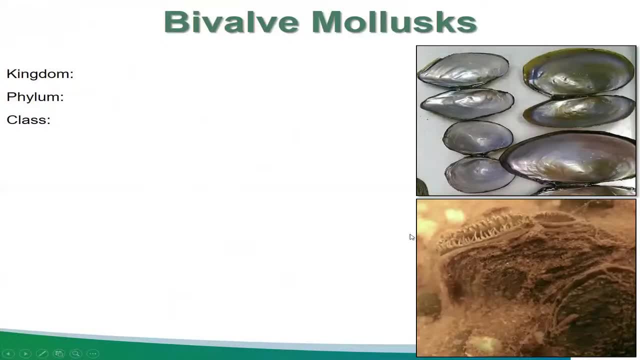 for these different species. So let's move on to bivalve mollusks and start real basic. So they're animals in kingdom Animalia. More specifically, they're mollusks, and not just any mollusks, but they're bivalve mollusks. 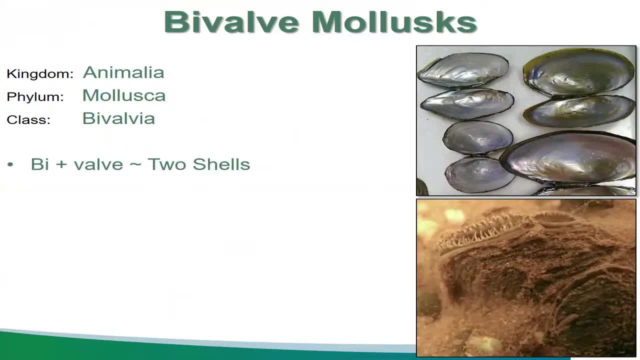 So they're in class. bivalvia And basically one of the easy things that I like to tell people is: a bivalve is two shells. right Bi is two, valve refers to the shell, And so these animals are two shelled organisms. 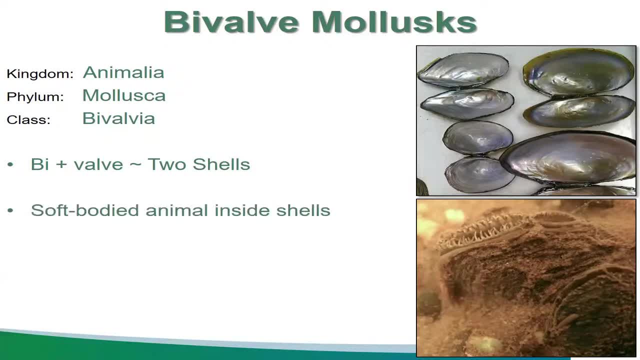 and the animal is actually the soft body that's inside the shells, So similar to like a turtle. the shell obviously is part of the animal, but there's a lot more behind the scenes inside that shell. One of the interesting things about bivalves. 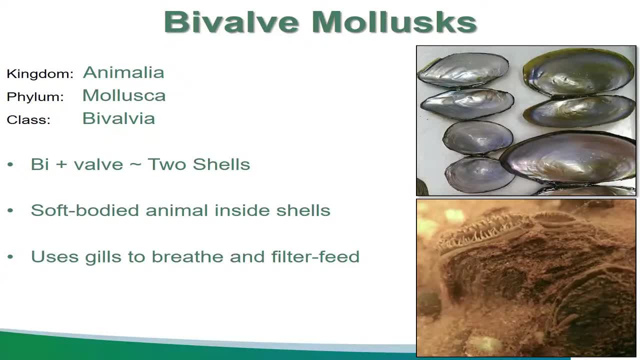 just like other aquatic animals is that they have gills to respire, to breathe. But they also use these gills to filter feed And usually the filter feeding bivalves will have bigger gills and multiple sets of gills. 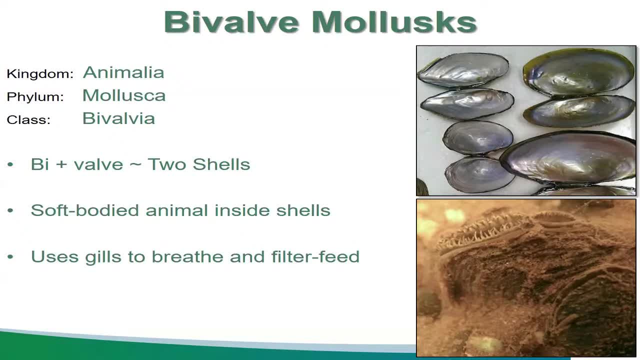 So they serve a purpose way more than just breathing, And we'll talk a little bit more about why those gills are so important. And just to kind of reiterate, we have multiple species all throughout the estuary and the world for that matter. 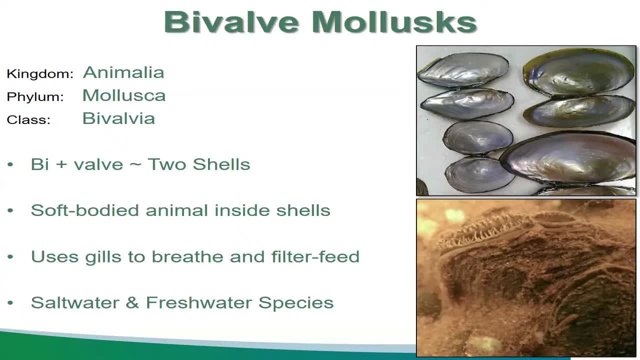 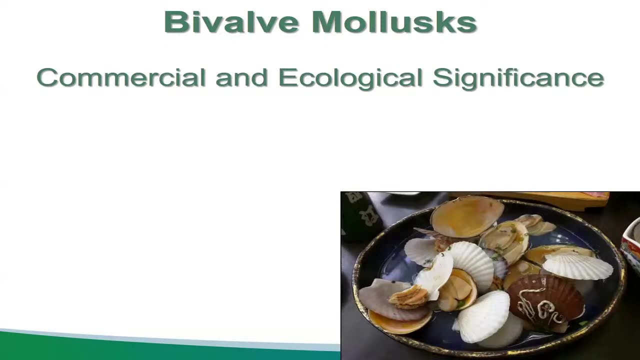 And they range from saltwater to freshwater species. There's brackish water species, And so they inhabit that entire range of tidal, non-tidal, freshwater and saltwater. They have a range of commercial and ecological significance, if you might not already know. 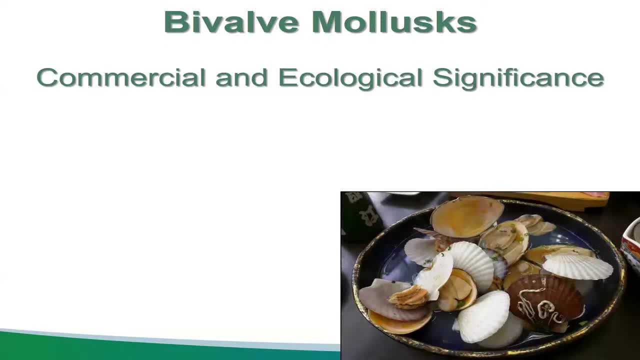 In the bottom left, you can see some clams and scallops on a dish, And so one of the main things that people get introduced to bivalves through is food. So if you happen to live on the coast or if you just like seafood, 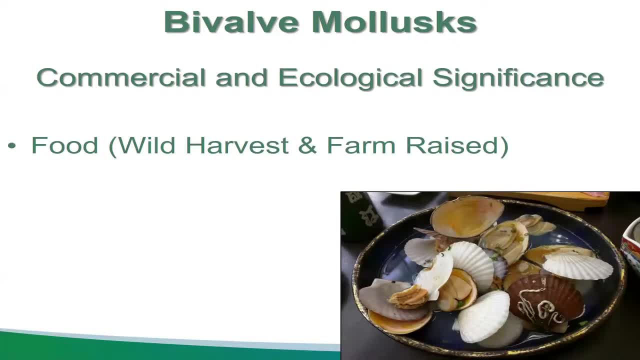 you've probably eaten a bivalve. We love to harvest them, We're really good at hunting them And we're also really good at farm raising them, And so farm raised bivalves generally. you hear of it every now and then. 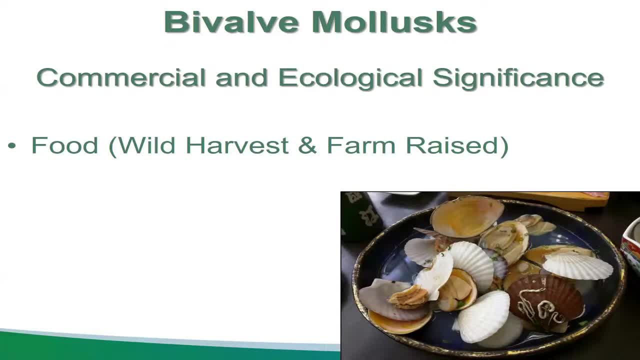 called aquaculture, And so one of the benefits of aquaculture- of bivalves and these kind of things link all together- is that because they filter water, it's actually kind of a good thing for the environment because you're adding bivalves to an area. 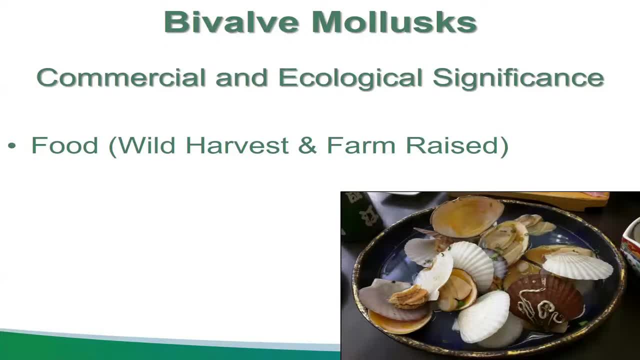 that would filter out some of the bad things per se in the water. One of the other reasons why we care about bivalve mollusks is for their products, So in addition to the meat which we eat, they produce things like pearls. Sometimes certain shells are valuable, whether for 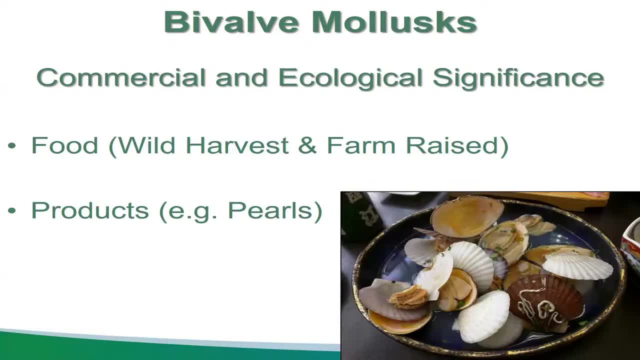 their aesthetics or for their function. Driveways paved with shell shells are used in the pearl industry. So there's a lot of other products, ancillary products other than just food And, of course, in addition to them just being really cool and we like them, they provide. 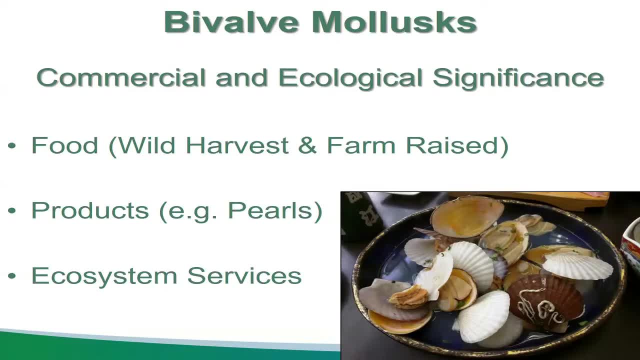 functional ecosystem services. So basically, they provide natural benefits to us as humans, as well as every other organism that lives in those environments, just by them being in those waters, And I'll touch upon these things in just a second So you can follow along with me at home. These are some of the well-known bivalves. 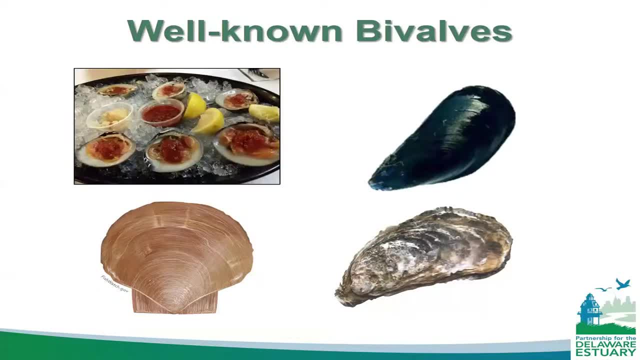 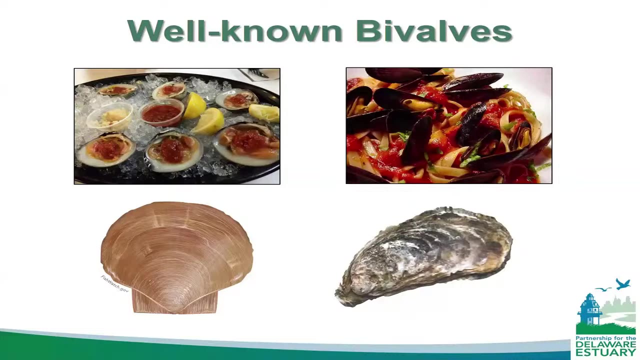 And so top left, it's clam, Top right mussel, Bottom left scallop and oyster. And what do we know about them generally? Well, it's because we see that we like to eat them, And even if we don't eat them, at least they're kind of iconic in the sense of what we see. a 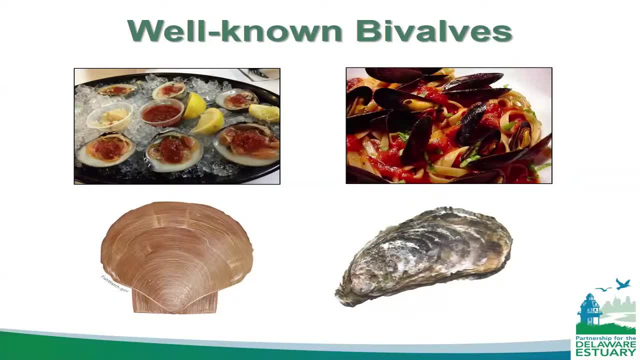 bivalve is, So it's food. We have the clams on a half shell, mussels, marinara, seared scallops. A lot of people don't realize the scallop that you eat is really just the adductor muscle and there's 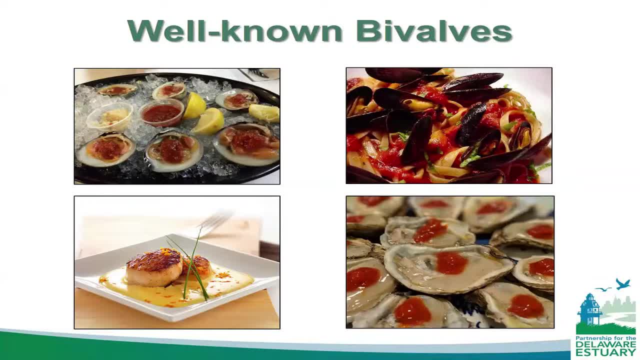 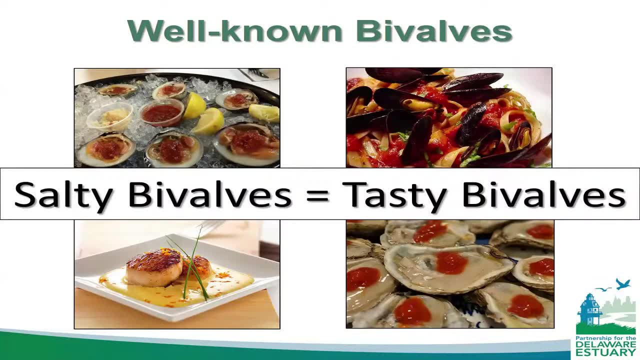 a lot more to it, And we have oysters- That's a pretty iconic one up here as well. So really, the take-home message is simply that salty bivalves are tasty bivalves. We don't eat freshwater bivalves, We eat the saltwater bivalves, And there's a number of reasons for that. But if you 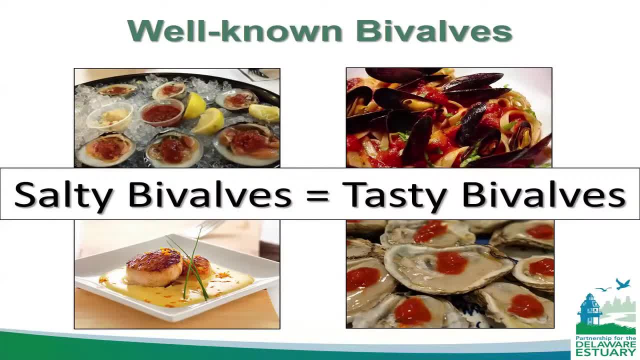 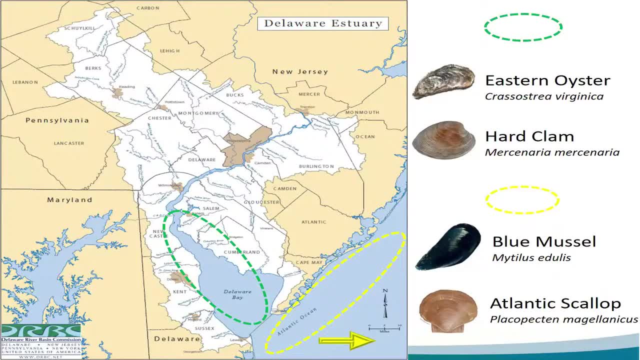 notice next time you go out to eat and you happen to eat something with a shell on, it probably came from saltwater, Just to hit this home. eastern oysters- hard clams. they tend to live in more brackish environments, so this kind of green hash line. We have oysters throughout the Bay. We have 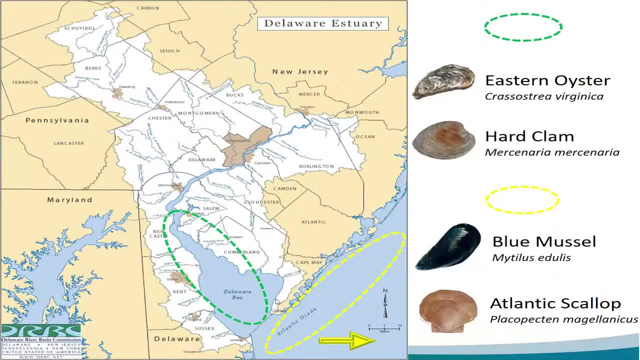 clams in the inland bays down in Delaware. Clams also live in these other bay areas and estuaries, And then we have blue mussels, which live in more salty waters, And of course scallops live a little more off the coast, But all these bivalves live in those salty areas Up here in these freshwater. 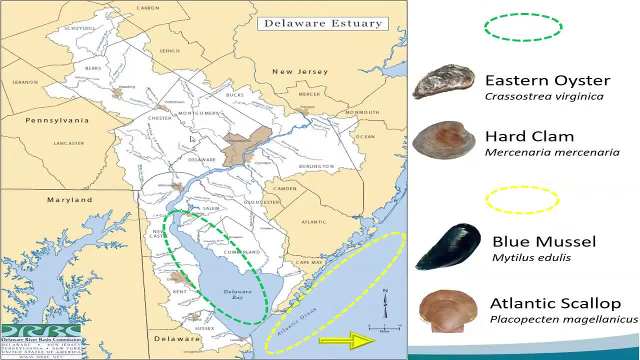 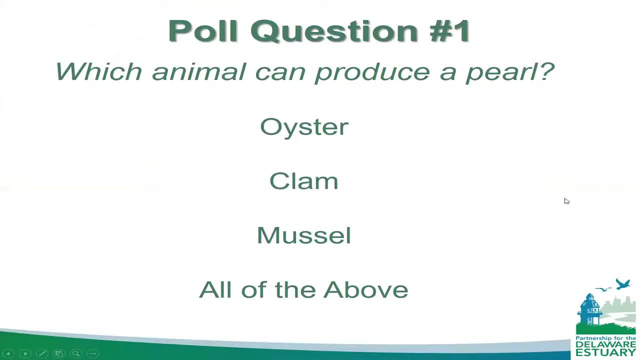 areas, you're never going to find those bivalves that you like to eat. It's just a different habitat. So here's our first poll question. So Leah's going to pop this up in a second: Which animal can produce a pearl? We got three choices, or maybe all of them. What do you think? 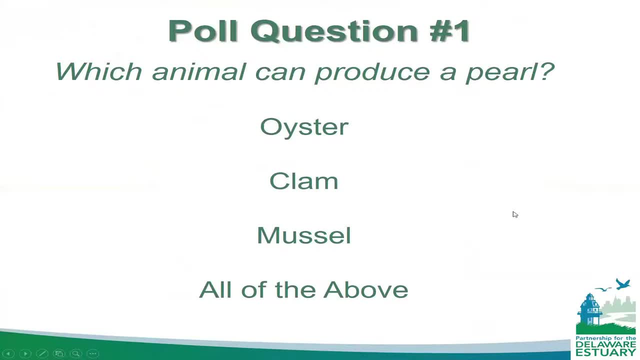 Notice. I really didn't say exactly which species, These are kind of general terms. I've seen a lot of oysters, That makes sense. A couple clams, All the above, A couple more seconds for everyone. Yeah, pretty much all the above, So it's a little bit of a. 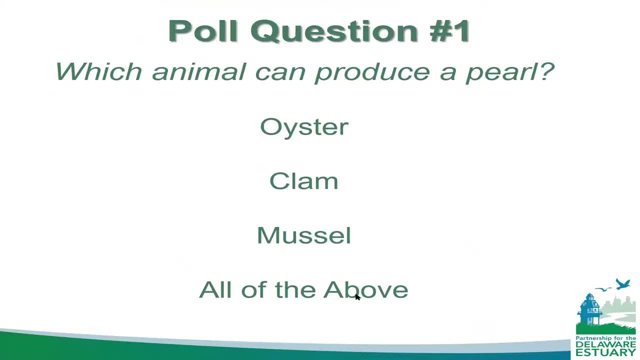 trick question, But really, a pearl is simply the bivalve's response to a foreign body that's in its body And so, unlike you and I, if we get a splinter or something, we can kind of pluck it out, If they can't open and close their valves enough to release that. 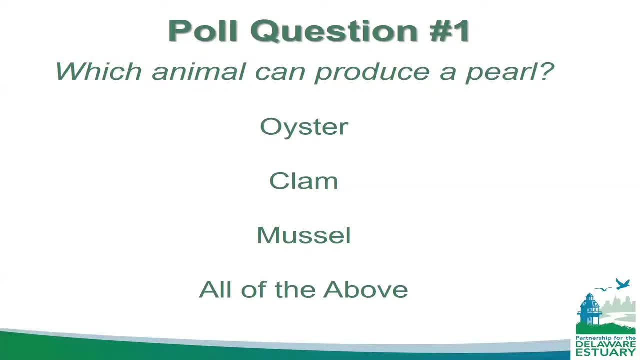 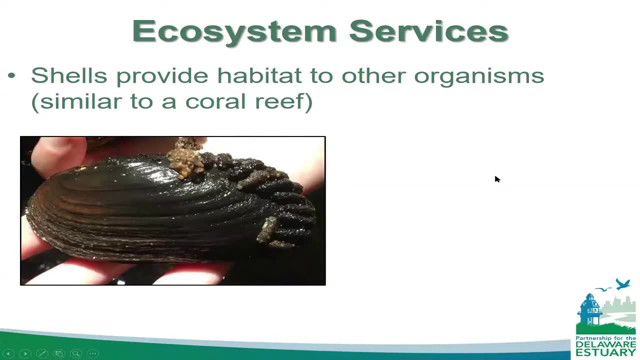 foreign body. it's just going to kind of encapsulate it. So that's what the pearl really is. So we'll move on All right. So back to the ecosystem services: Bivalve mollusks. most of these, then have shells that serve as habitat for other organisms similar to a coral reef. 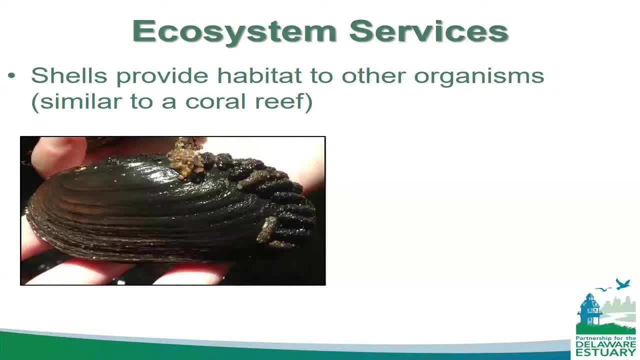 not exactly the same, but the concept is similar. So on the left we have a freshwater mussel, and macroinvertebrates like to lay their eggs on mussels, And so this is kind of important where, if you're in an environment where there's only sand or maybe even silt or mud, those shells 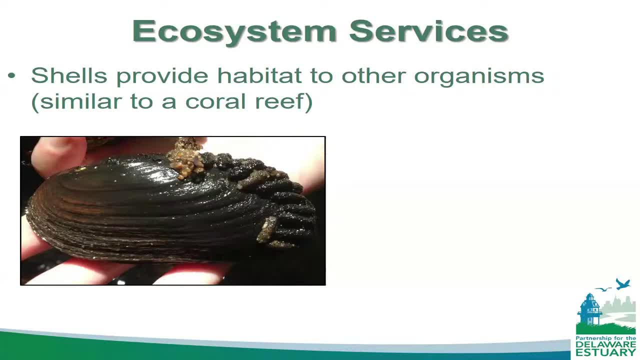 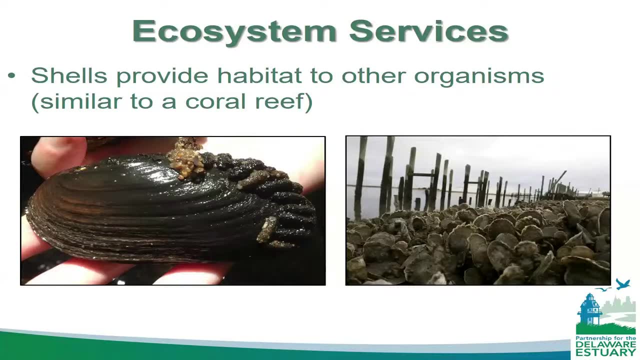 provide that rigid, hard structure. Animals also like to hide in and amongst those different bivalves. So for example- this is a really good example- is oyster reefs. So oyster reefs, in addition to providing vast amounts of oysters, they're providing all that space and kind of almost. 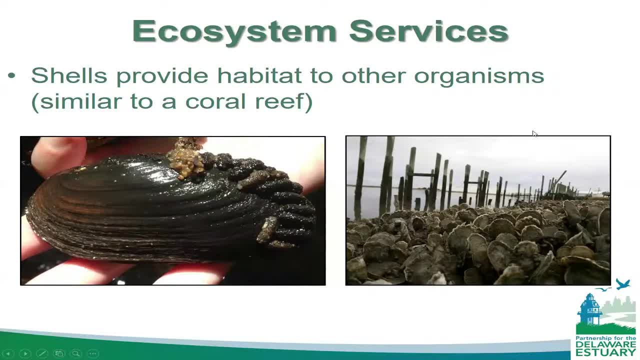 like a playground for all of these different fish to survive and live in, in addition to all the things that like to eat those fish. So it's kind of supporting this greater ecosystem beyond just the oysters alone. Getting back to the whole gill of the 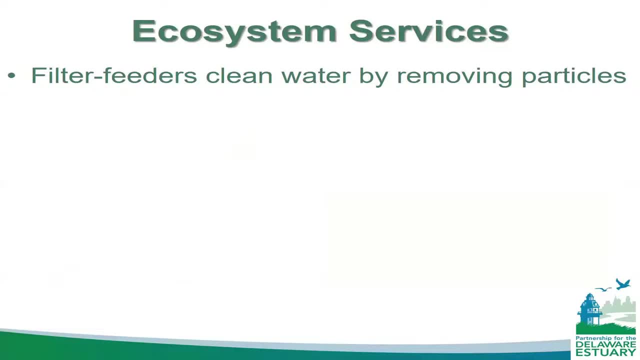 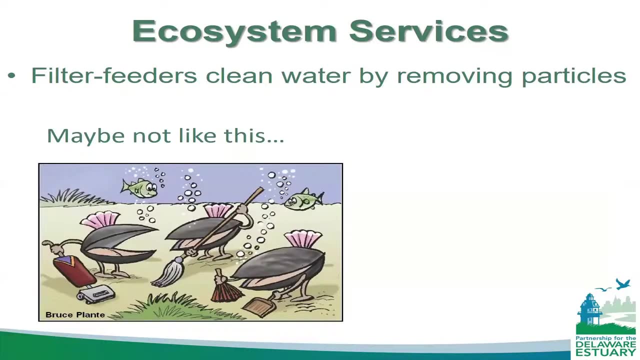 mussel of the bivalve player is all about making sure that you seal and save Earth, because I really think there's a lot of different, different parameters that a monocular and living creature care tank can��면, has or can actually do. So let me start off with You Dig into one of 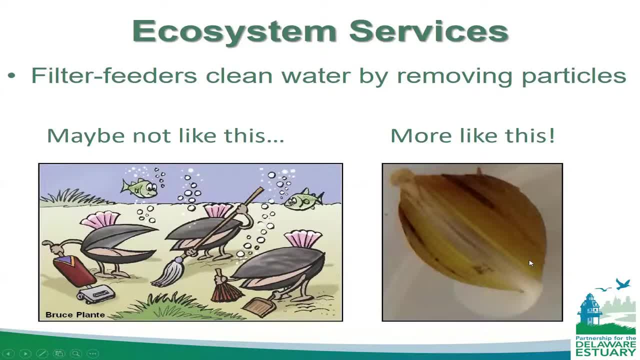 your ocean coverings and see what all the outdoor sites do, and you'll point to what that explain in a moment. I'm just going to start with sort of with another one, but I think that the community of bivalves actuallyagonizes with summer fish floe and 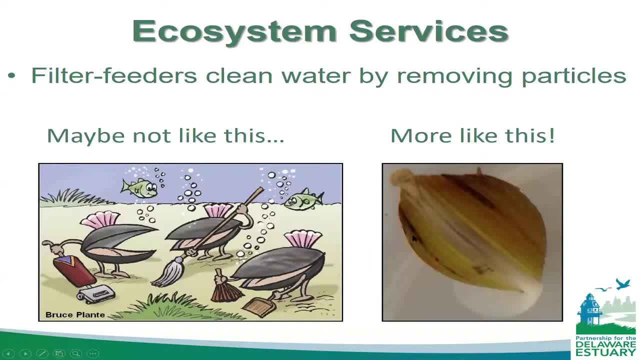 far more central hot spring wetland. So what we seem to do is sort of put some of those they're doing is they're stripping out really fine particles, eating what they want and rejecting what they don't, But just by them feeding and living in water. 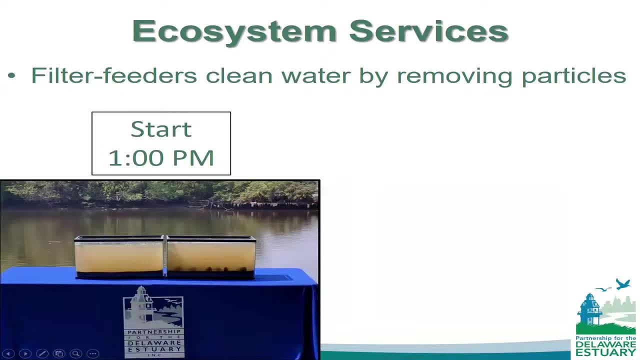 they're clarifying the water, And so one way to look at this is if we put two tanks next to each other with the same river water, we have mussels in one tank and nothing in the other tank, and they both have sediment After about an hour. 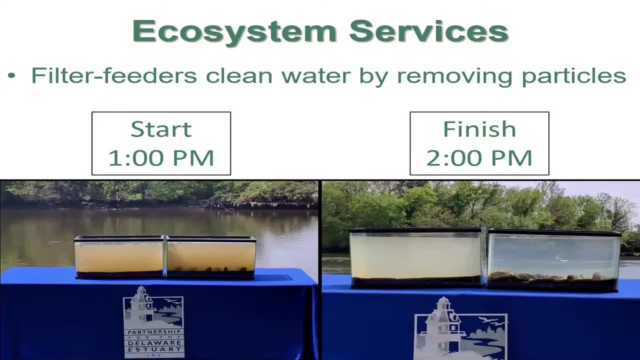 you can see that both tanks are a lot clearer, and so the right one is more clear than the left one, though, And so the the difference is that all the really big particles settled out regardless. That's why the left tank looks a little bit lighter, but it's still really murky, And so if we zoom in that, 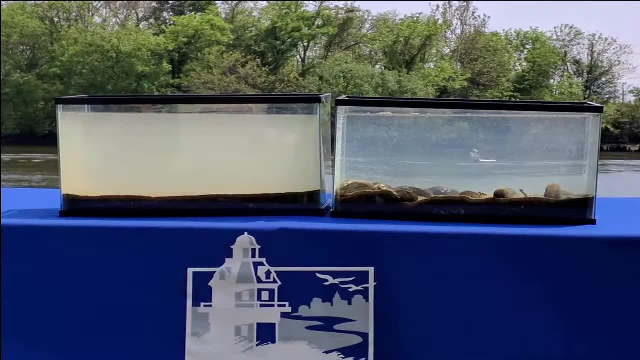 murkiness is really all those fine particles, bacteria or anything below, let's say, a hundred microns, so you know, not even a millimeter in size, really small particles. Those animals effectively ate all that material and that's why you're seeing a lot of murkiness. 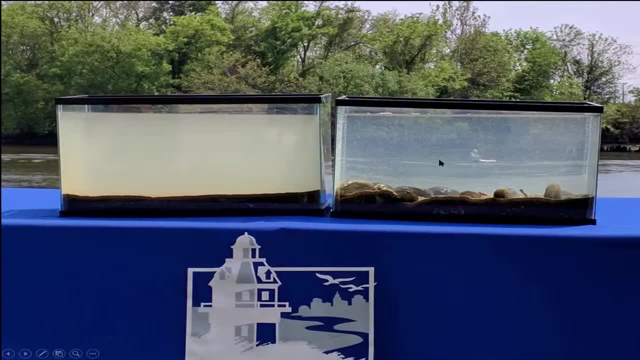 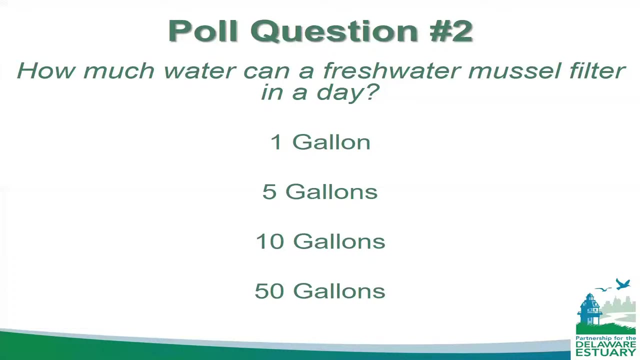 So this is kind of an easy demonstration to show that, hey look, these mussels are actually filtering out things in the water that really just stay in suspension. So on to our second question related: how much water do you think a freshwater mussel can filter in a day, And this isn't exactly a hard answer. but 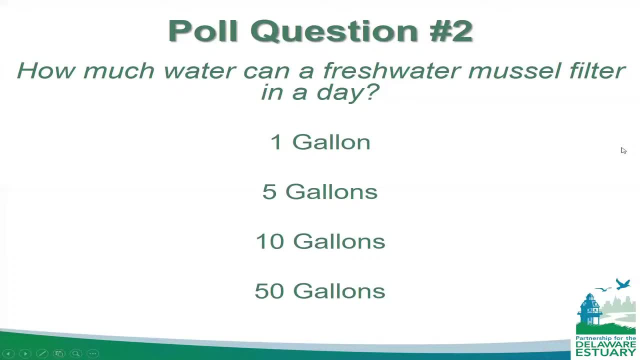 generally how much you think, And it depends on the species, it depends on the size, it depends on the water conditions. Two: much food, too little food. looks like we're trending towards 10 to 50 gallons And yeah, so yeah, generally we say we'd like to say about 10 gallons. however, 50. 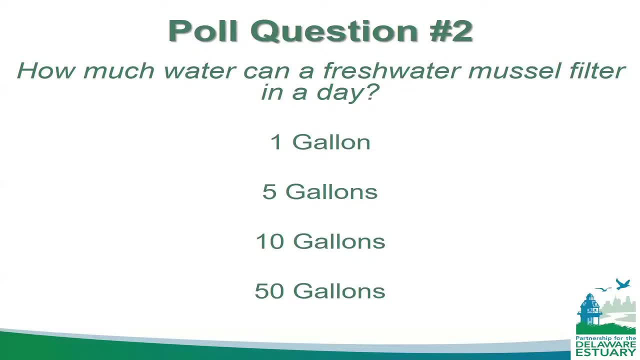 gallons. it could be a bit of a stretch, but again it depends on the species. There's some species out in the Mississippi and other drainages where they can approach, you know, almost like a dinner plate size, and just to meet their metabolic demands hands they're going to have to process a lot of water. So good job, guys. All right, let's move on. 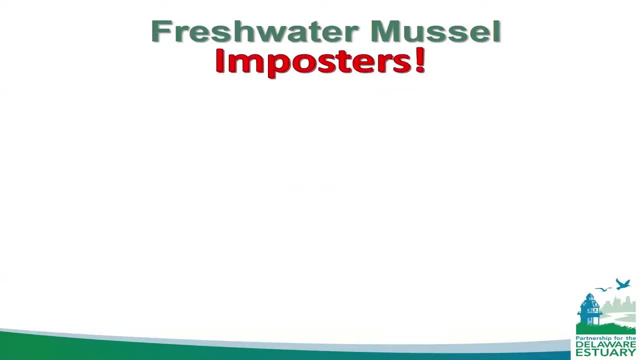 So let's talk about freshwater mussel imposters. These are all freshwater bivalves, but they're not quite what we call freshwater mussels. The first one is a pea clam, also called a fingernail clam, And these are native. They don't really grow beyond the size of your fingernails so aptly. 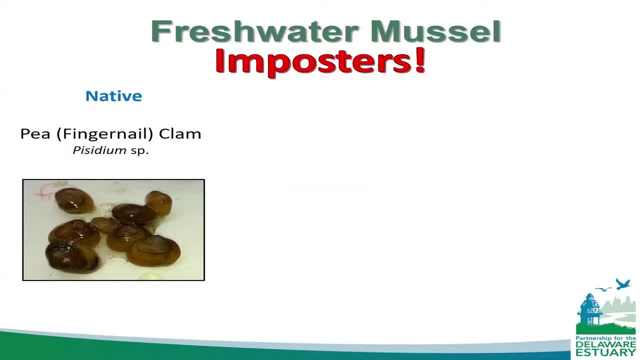 named, And so they're not freshwater mussels, but they do live in our freshwater systems And I'm not going to talk too much about these. I just wanted to mention them. So another one is the Asian clam. I mentioned it before. It's non-native, but it is here And you probably 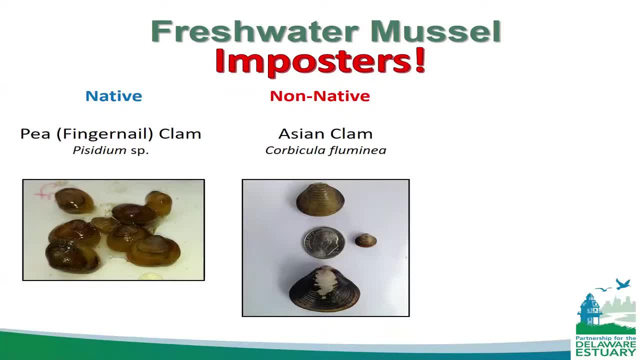 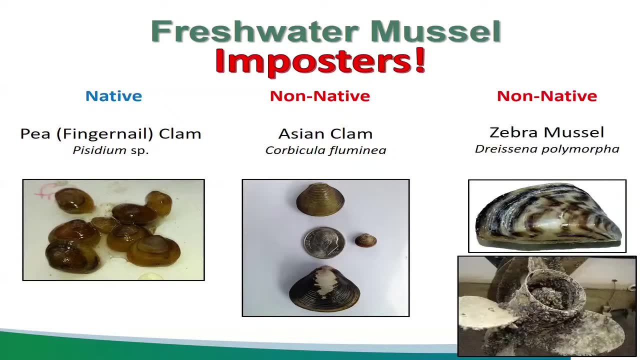 have seen its white kind of bleached shells on if you stroll along any freshwater stream or river. they're pretty ubiquitous. And then, of course, the zebra mussel. So most people usually know about the zebra mussel. Some people will know about the Asian clam and that'd be pretty impressive to know about the. 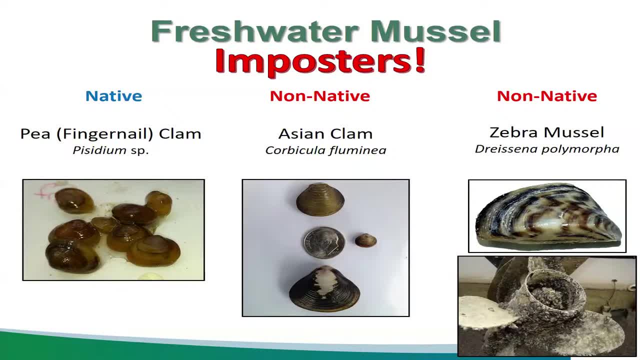 pea clam. But again, zebra mussel is a non-native species. It tends to biofoul a lot of things. I won't talk much more about these guys, but just know that they exist and they're not mussels. 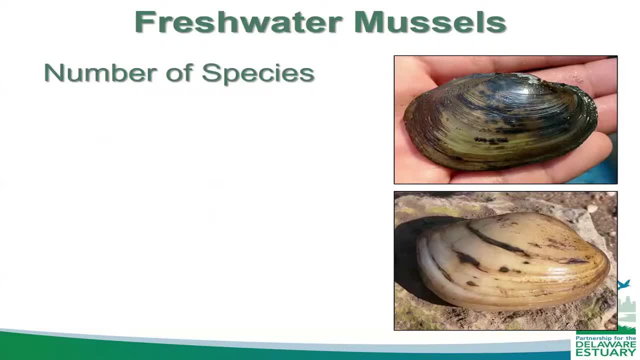 but they do live in freshwater. So let's get on to our freshwater mussels. We have about 700 species worldwide and that's kind of a lot of species with over 300 in North America, So we have the most species of any continent. 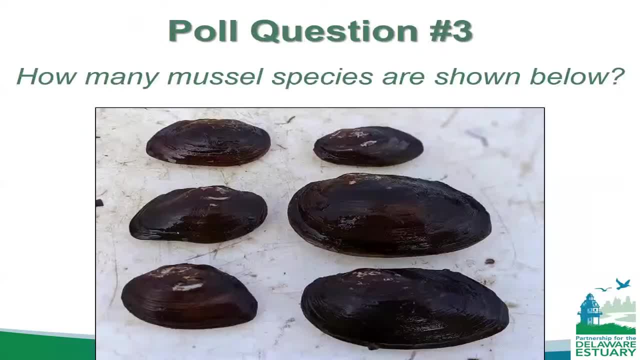 And locally we have a little over 10 species in the Delaware estuary. Third poll question. So we're going to take a second and look at this photo. I told you there was about 10 to 12, maybe- species in the Delaware estuary. How many species do you think are in this? 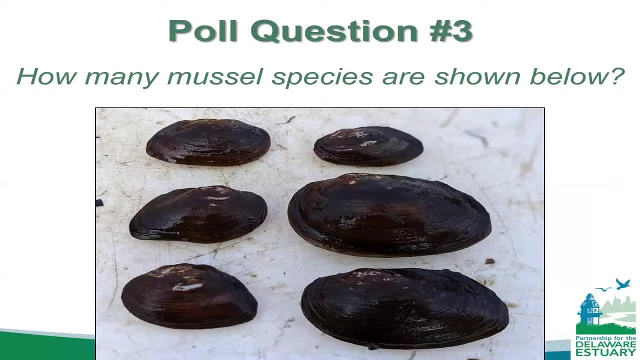 photo. It's kind of all the same color, but the shapes of the shells are a little different. So give it a second and tell us what you think. One, two, four, six, Wow, All over the place. That's good, That's exactly what I wanted. Four, All right, So yeah. 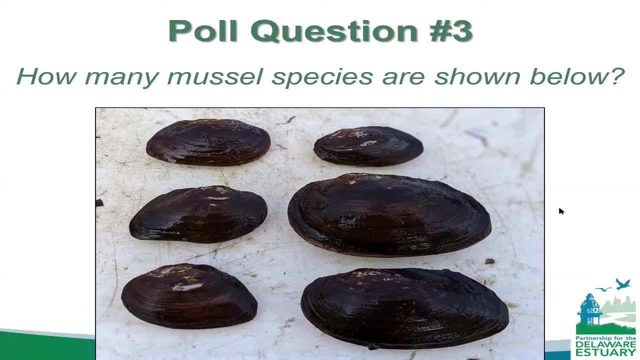 kind of a trick question. They're all the same species, But I can see three or four potentially. The shape of the shell is really reflective of how it was grown, And so suffice to say freshwater mussels are really flexible in the way that they grow. Sometimes they'll look. 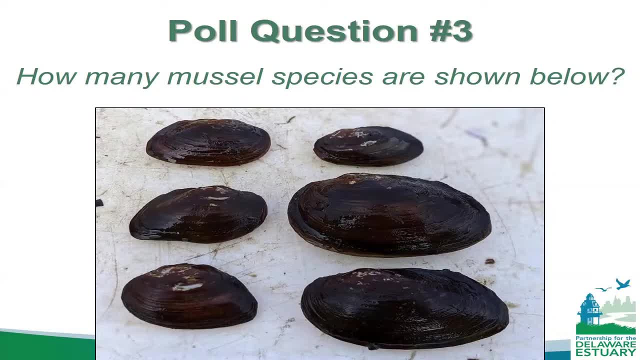 completely different. Sometimes they'll look completely different. Sometimes they'll look different shells, different shapes, different colors in different regions, but they're all the same species. So it's kind of a cool thing that mussels do, So let's just introduce some of the 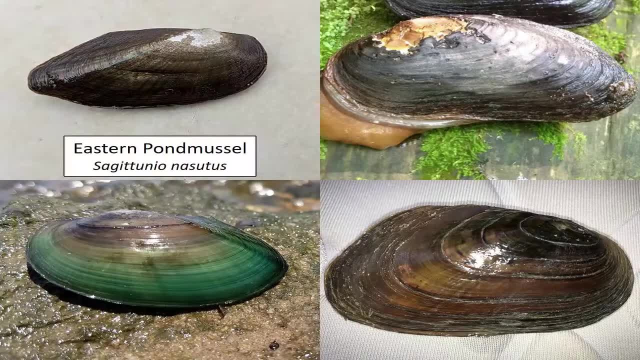 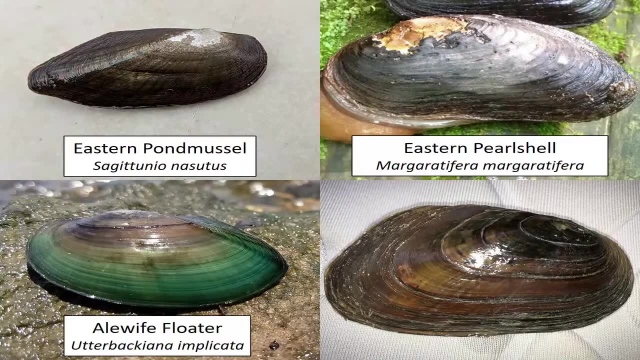 mussels that we have in our estuary. Top left we have the eastern pond mussel, Top right we have the eastern pearl shell, Bottom left we have the alewife floater And bottom right we have the eastern elliptio. So these are all kind of like you know, maybe weird names to some people. 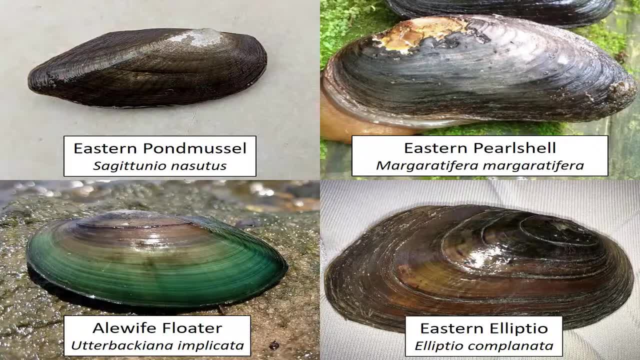 Sometimes they're kind of cool. But really if you look at the shells you know there's all kinds of different colors, different shapes. This one has this kind of tip at the edge. This one I like because it's almost like a boomerang or like a banana, almost It has this indentation right here. 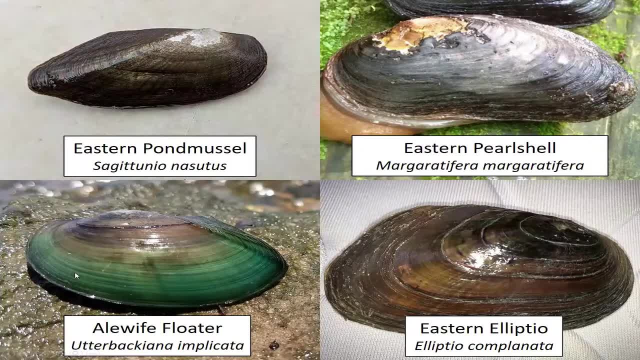 Interestingly, this alewife floater here it's very nice, emerald green along the ventral margin, So along the bottom of the shell. And this is actually the same shell, same species of that photo I showed you before. So you know, really dark black shell versus 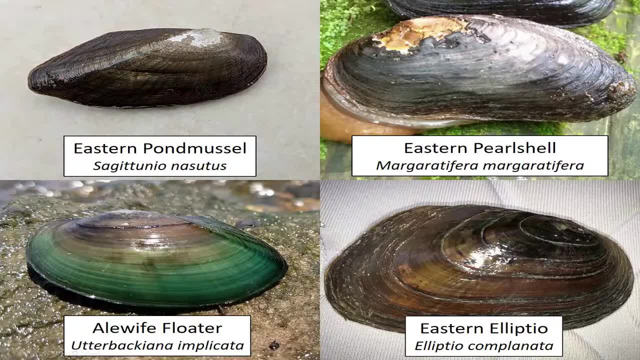 emerald green. You know, it's just where it's grown. And even where it's grown you can have green, red, yellow, brown of all the same species. Eastern elliptio: here we have this kind of nice bands of rings. The rings. you can't necessarily age the mussels, but it's certainly. 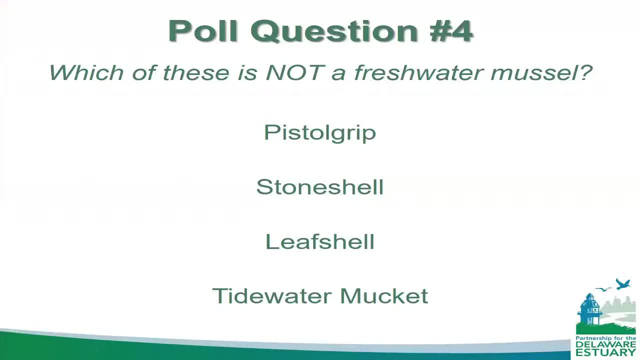 an indication of the conditions in which it was grown. So here's our last poll question. It's kind of the names we said before. which is not a freshwater mussel? We got pistol grips, stone shells, leaf shells or tidewater mucket. Give you a second to say that. So it's not a. 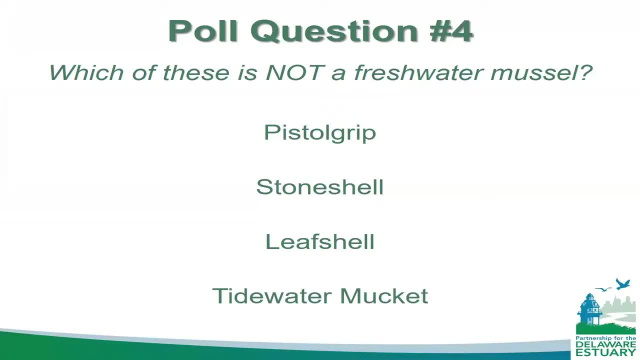 freshwater mussel. We got tidewater mucket kind of leading right now. Be curious what you guys think. Let's give it a couple more seconds, All right? Man, not a freshwater mussel, tidewater mucket, All right. So let's stop sharing the poll. 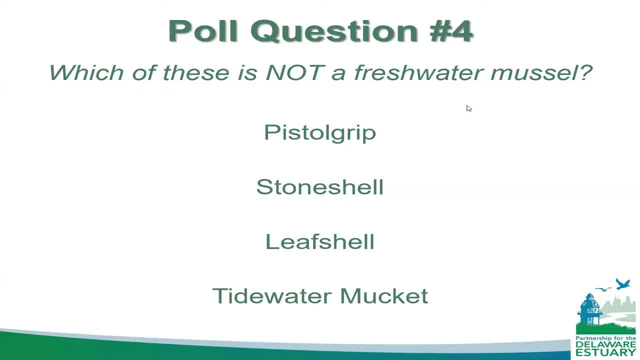 And I'll say that, first of all, the pistol grip is a mussel And that's what there it is right there, Not native here, but it is, And you can kind of see it's kind of resembles a pistol grip here. 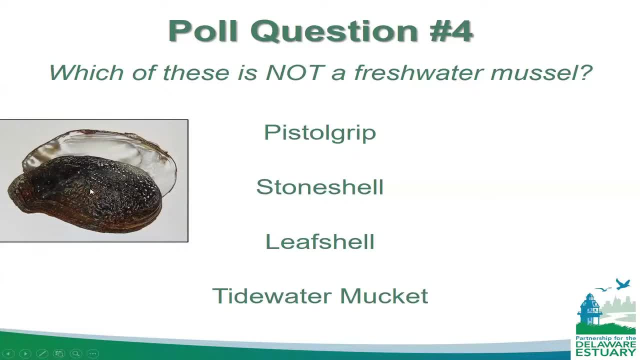 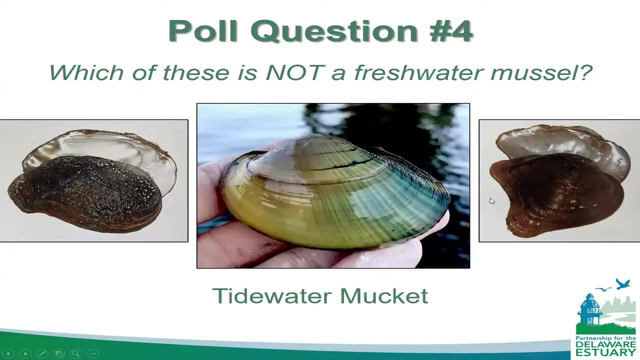 with that kind of dimpling and it kind of extends a little bit. Then we have the leaf shell, And so this is considered extinct. But again, this is a true mussel. You can kind of see it almost looks like a leaf- certain leaves- And then of course we have the tidewater mucket. So yes, 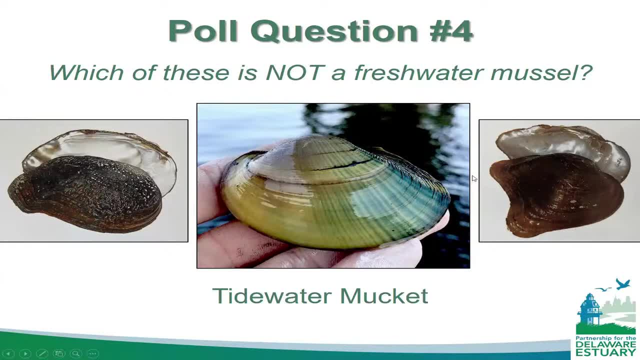 the tidewater mucket is actually probably our signature species of the Delaware estuary. It uniquely lives in tidal water. The stone shell was the correct answer. Stone shell is made up, So the tidewater mucket we have is kind of nice yellow, with these green to blue bands or rays that. 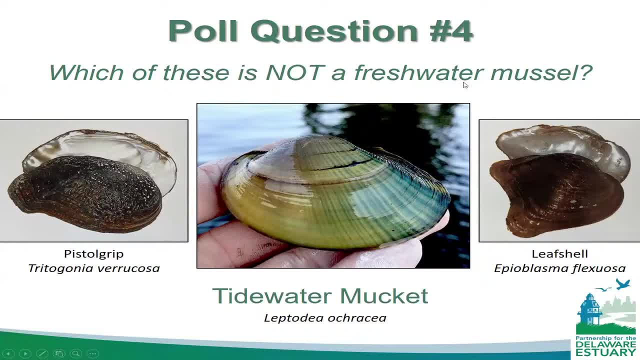 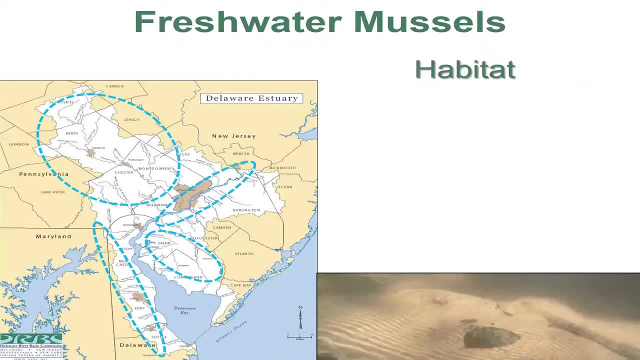 extend off of it And so, yeah, like I said, they only live pretty much in fresh water and, I'm sorry, tidal fresh water. So we have them throughout our estuary In the tidal portions. So where do these mussels live So well, it needs to be fresh, right? So 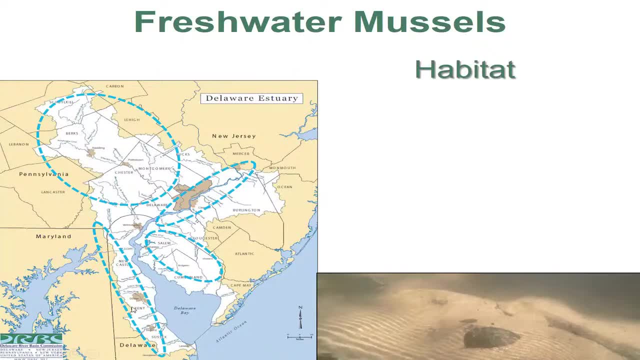 pretty much all these areas, that's not these salty areas, All the tributaries and everything else. And so what I'd like to say is: you know, bring it back to the first principles and basics of what it needs to live. So it needs to be fresh water, There needs to be oxygen in the water. 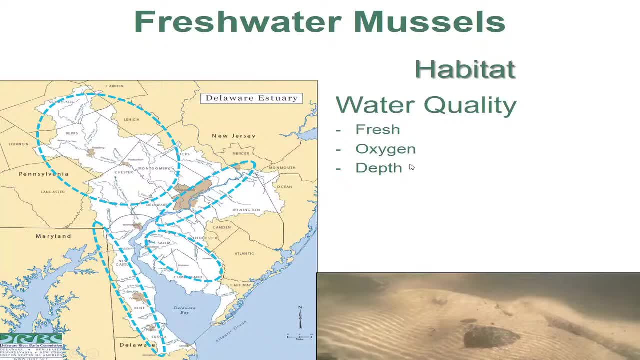 Can't be just kind of a stagnant swamp. It needs to have enough depth so it can't freeze in the winter And it can't dry up in the summer. So, beyond that, where do they live? Well, they actually live in the substrate, under the sand and mud and clay. So so long as that. 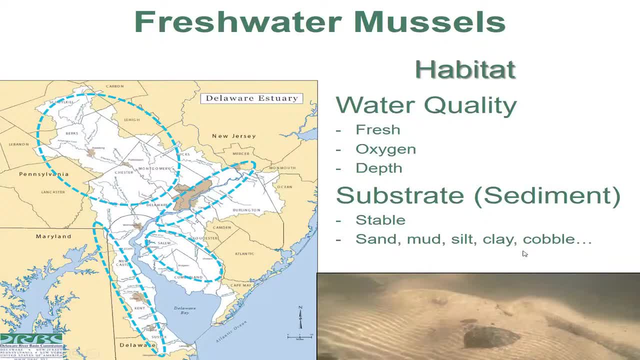 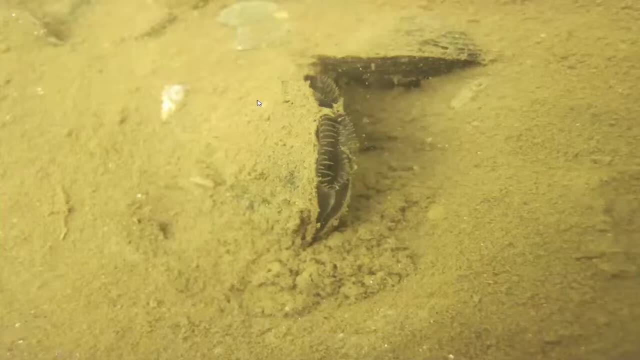 substrate is stable, they'll live in it, And they can live in all kinds of different sediments, And sometimes it depends on the species, but other times you can have very generalist species that will live in sand, clay, silt, cobble, you name it. So here we go, Just as an example. 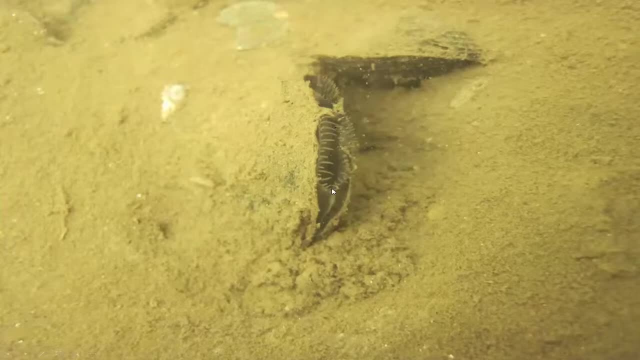 we have the Eastern Ellipteo here. You can see its cilia pretty well. Took this picture a couple of years ago, And so this is the inhalant siphon, So that's where water goes in, And then the exhalant siphon, where water goes out, goes that way, And so there's another muscle here And, as a 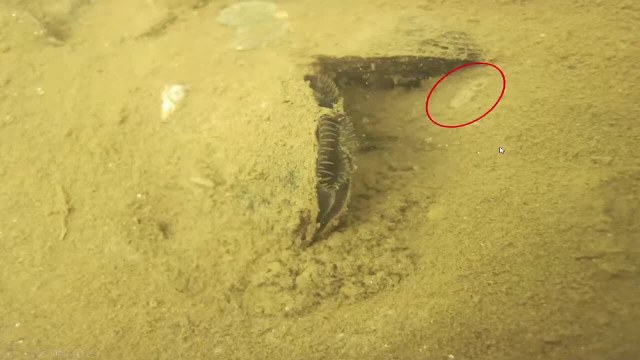 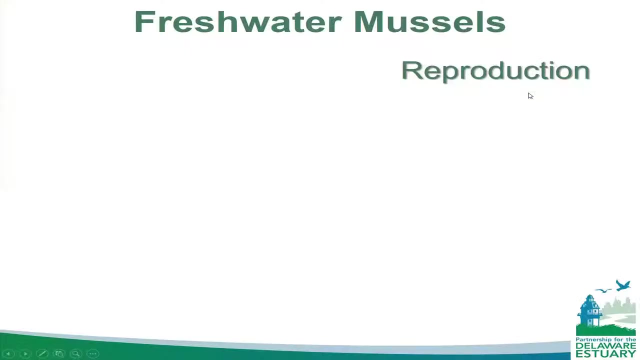 bonus for those with keen eyes, you may have already picked up: there's actually an Asian clam right here, And so same deal: Inhalant siphon right here. exhalant siphon right there, All right. So the most interesting thing about freshwater mussels- probably the 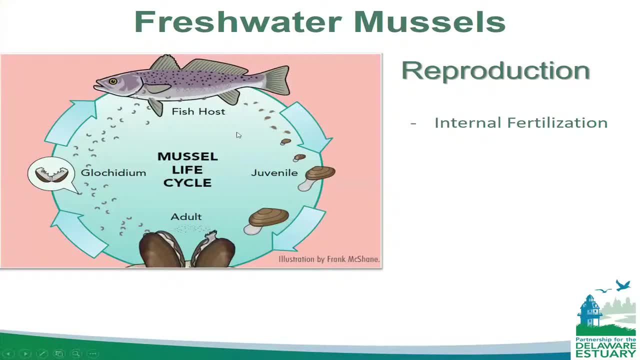 most interesting thing about freshwater mussels probably is their reproduction. So to keep it short, they fertilize internally, which is rare. So most bivalves are broadcast spawners, The sperm and eggs go expel into the water, column tides and currents take care of. 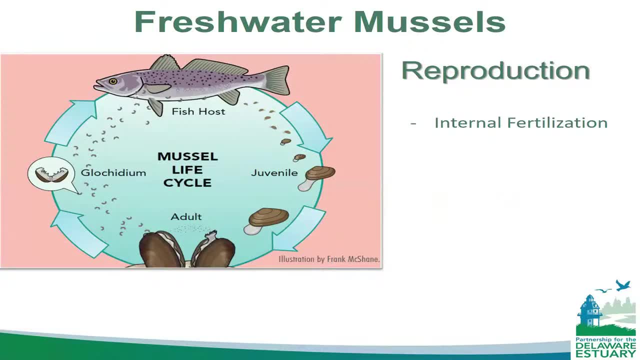 everything else. These freshwater mussels remember. most of them live in non-tidal streams one way, So if everything goes up, everything goes downstream. eventually you're not in the stream. However, these freshwater mussels have been able to adapt, And so males release sperm, females take. 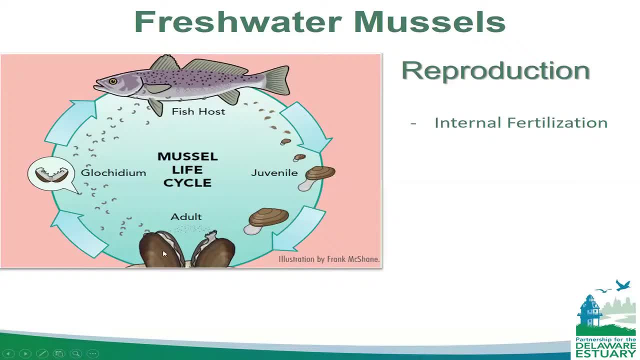 in the sperm and fertilize their eggs internally. So they have control, They're keeping their glochidia inside of them and they're waiting for a fish host, And so this is another fascinating part of their life history. So these glochidia, these kind of Pac-Man type larvae- 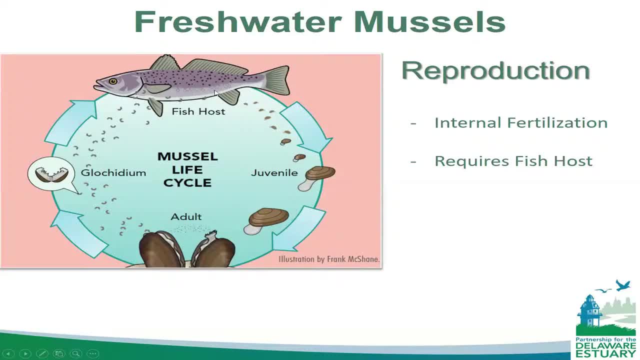 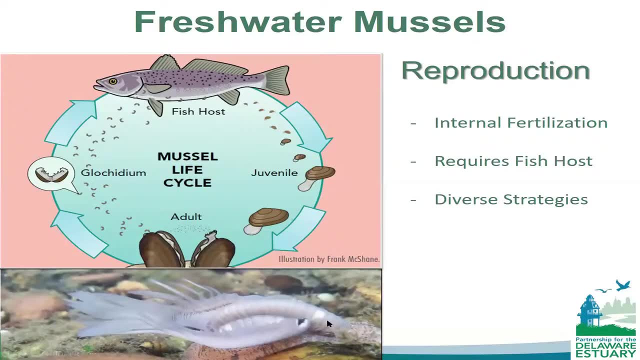 need a fish host to reproduce. Once they attach to the fish host, then they'll settle out, And so there's all kinds of diverse strategies to kind of lure that fish close by. This is a lure. right here We can see there's an eye spot and these are actually just. this is part. 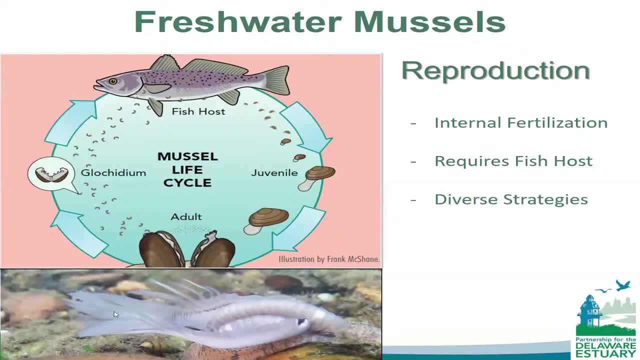 of the muscle. However, it kind of looks like a fish where you have these caudal fins here and you have some of the dorsal spines here. This is the glochidium here. This is actually a Eastern elliptical glochidia And you can see these kinds of spikes or spines, fangs. 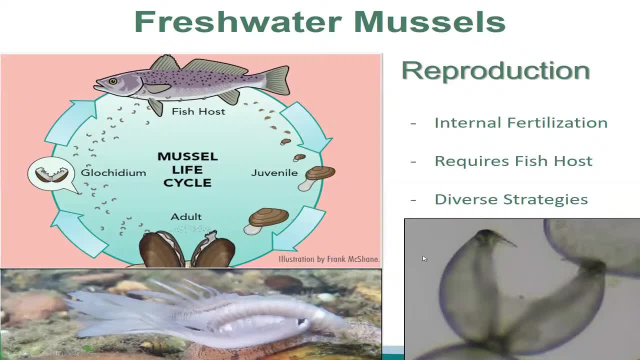 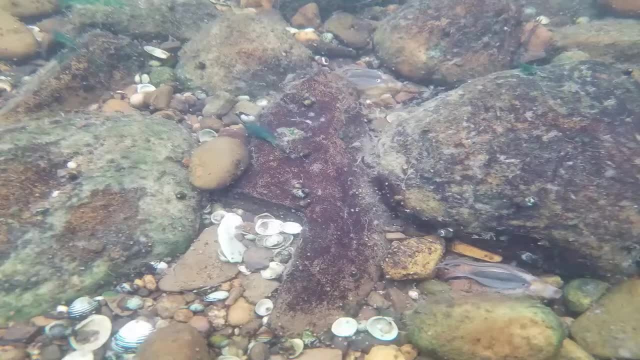 if you will, that can actually latch on and help it secure itself to a fish gill. So if you could see here there's actually two muscles displaying right there, And so what you can see is there's an eye spot there, an eye spot there, same deal here. 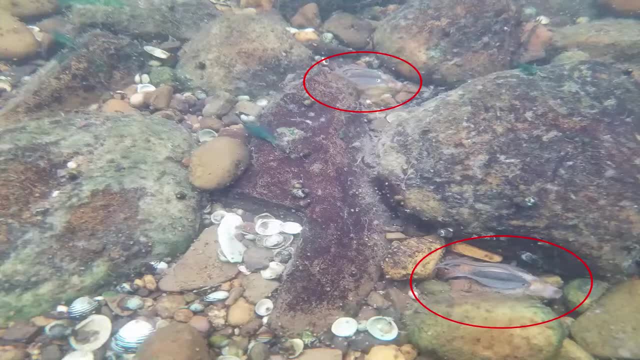 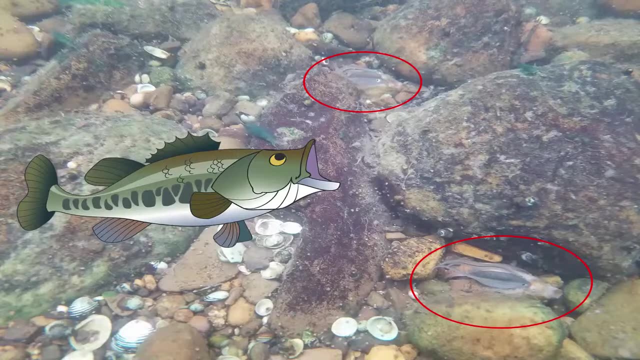 And the general idea is that those that look really promising is probably going to attract things like a largemouth bass, And so if Mr Bass here finds one of these lures and says that actually looks like my lunch, it'll actually go close enough. maybe try to bite it. And if it, 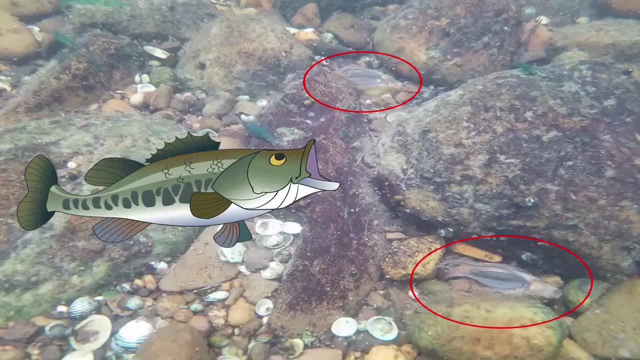 bites it, it's going to break open those gills that are full of those larvae and the larvae are going to get close enough to attach to the gills. So if it gets to attract the bass enough, then that muscle is able to reproduce. If the lure is not really good, it's not convincing, it's probably. 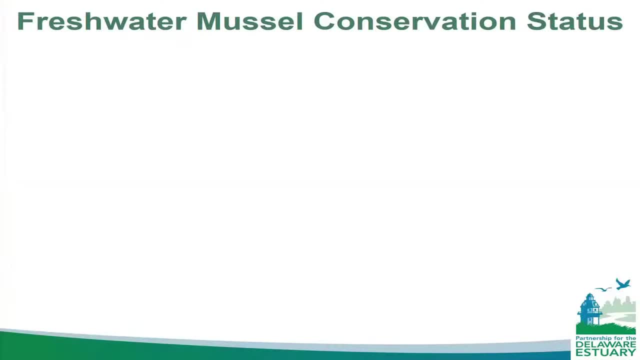 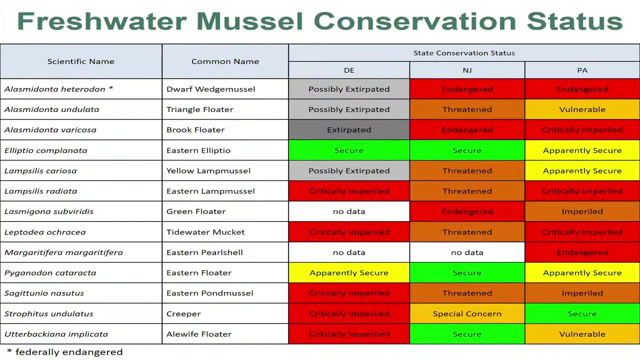 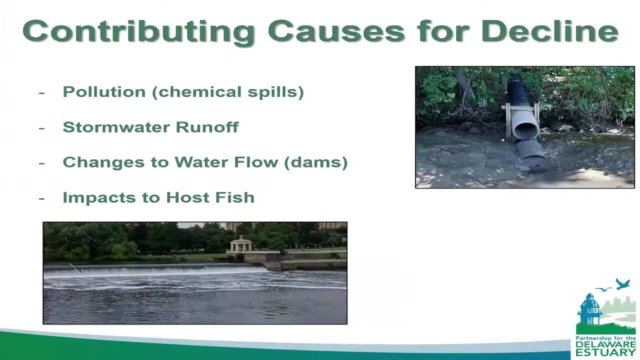 not going to reproduce. So a bit on conservation of muscles In a sentence. it's not so great. There's a couple of generalist species that are doing okay, but generally there's a lot of declines, both locally and nationally, pretty much worldwide really. So there's no one main. 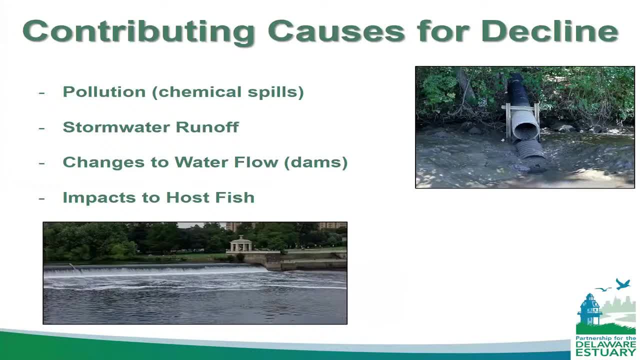 reason for decline. However, these are some of the reasons that seem to be contributing in a proportional manner. So we have pollution. pretty simple. If there's a chemical spill and it kills everything in the area, well, guess what? It killed the muscle. 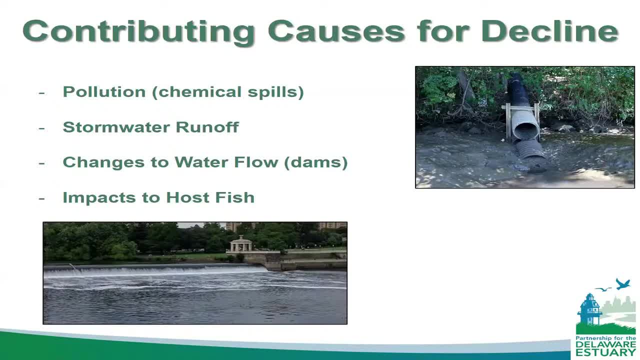 too. Stormwater runoff is another one where there's increased flow into our streams. It's going to disrupt the habitat. Remember, they live in the mud, in the sand. So if the sand is moving, well, they're moving too. Changes to water flow If all of a sudden you put in a dam. 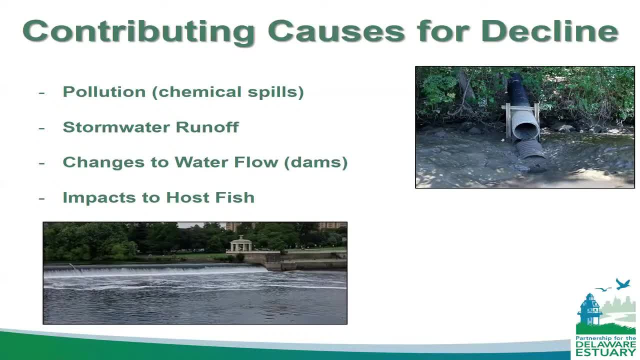 and the water flow drops, muscles are uniquely adapted to live in all kinds of different waters. In addition, those dams impact fish. So the less fish that get up to the water- sorry, to the water, the muscles that live in that water- you have less fish host to reproduce. So getting back to 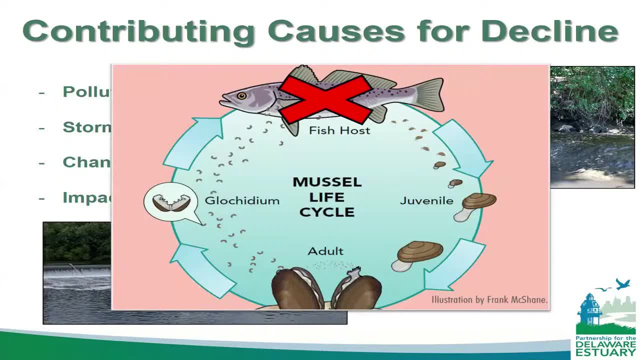 our life cycle. if you get rid of that fish host, there's going to be a problem. You're not going to be able to get to the juvenile stage, to get to the adult, And so that's what we see a lot of times is. 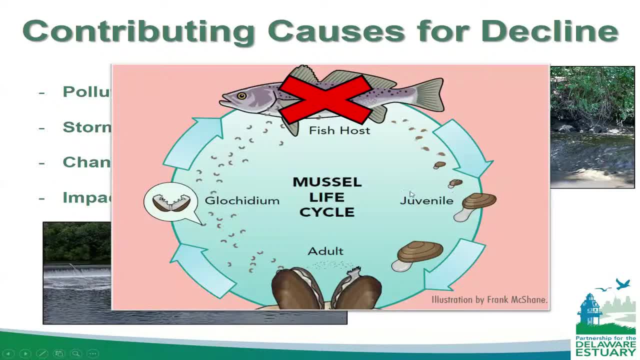 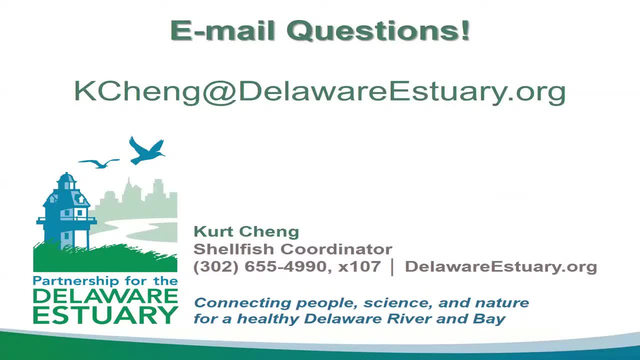 only the adults survive, and we don't see juveniles In a healthy population. you want both, So that's it for me. I went a little bit over and I think we're a little pressed for time, but I'll answer any questions now And, if not, feel free to email me, kchang at delawareasteryorg. 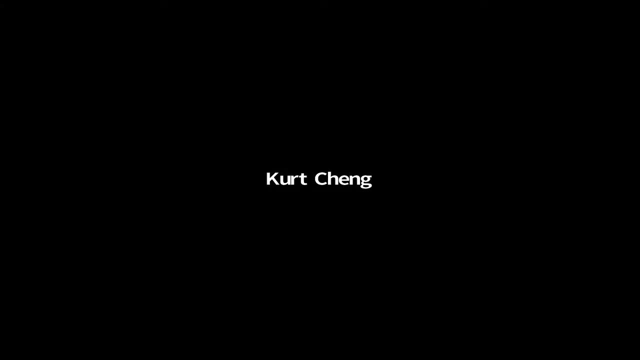 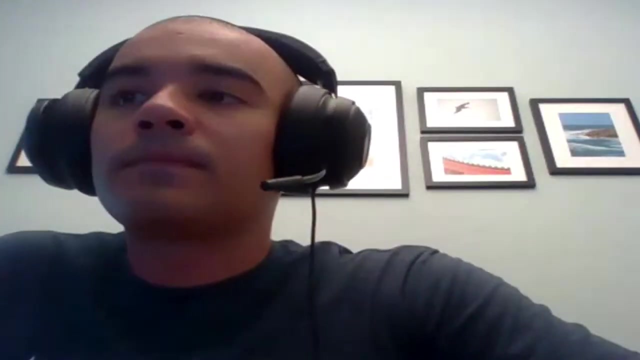 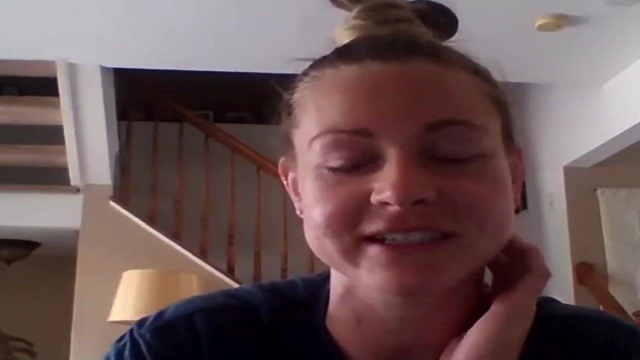 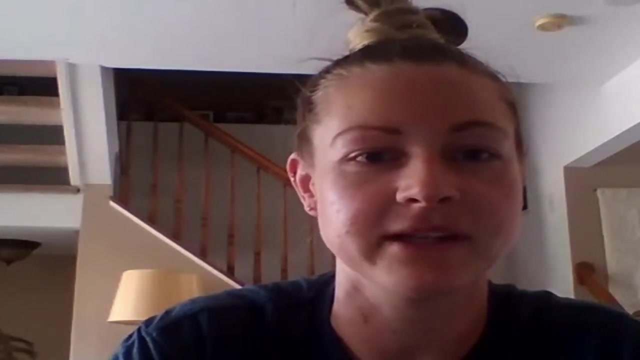 I'll be happy to answer any questions. Emily is muted. Thank you Appreciate that, Kurt. Thanks, That was a very ali- informative freshwater mussel presentation. So we do have about maybe five minutes or so to ask Kurt a few questions. if you know, folks want to type them into the Q&A box. We might have had a. 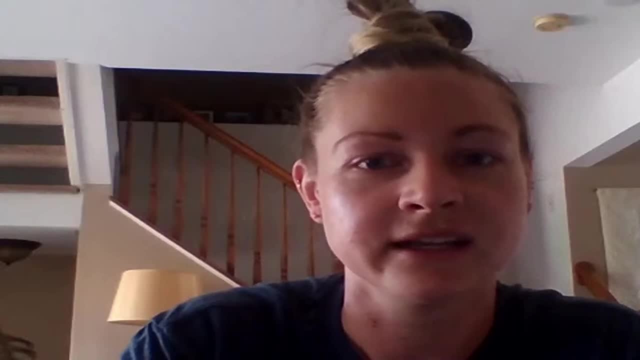 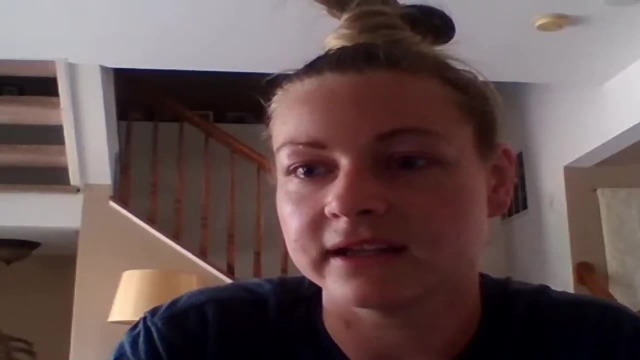 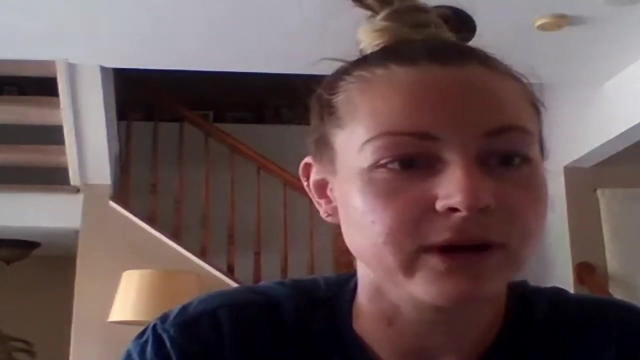 few come through already. so let me take a look and if we don't get to all of the questions, you can follow up with Kurt in an email and I will put his email in the chat box right here so you can see that if we don't get to everything. So we did get a couple questions about freshwater clams. 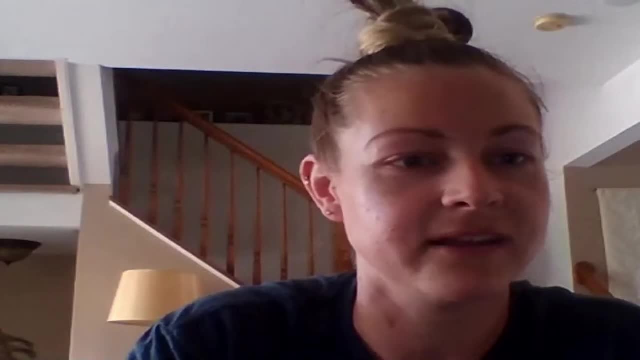 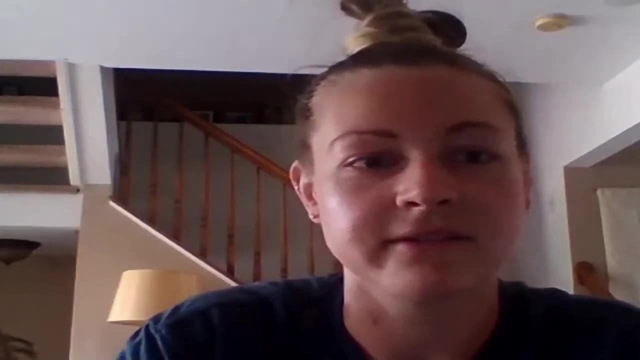 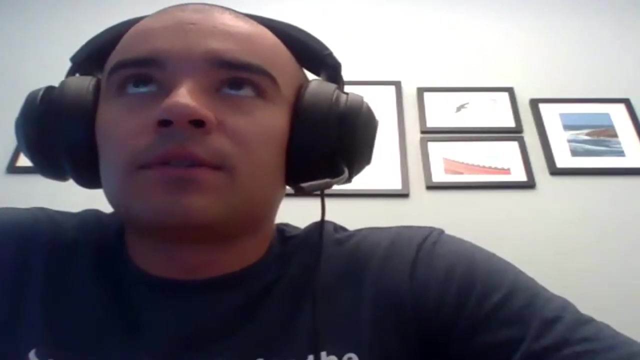 actually So one was. I see people in the Schuylkill River around Norristown harvesting clams and assumed that they were eating them. Do you know why they are harvesting them? Yeah, so the quick answer is that it's a food source. In other countries it's a common. 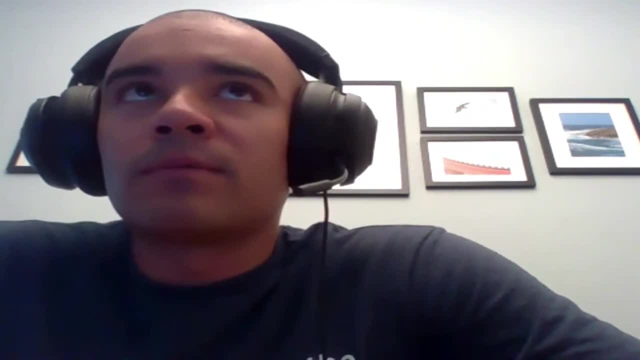 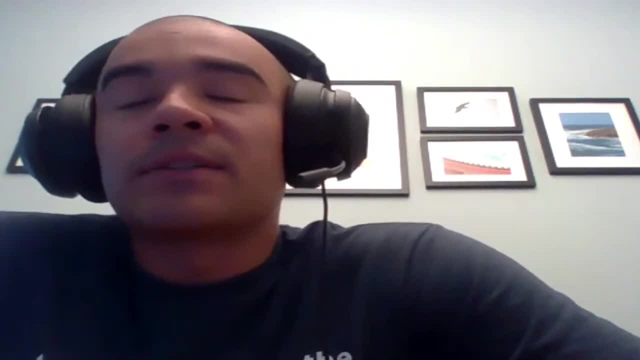 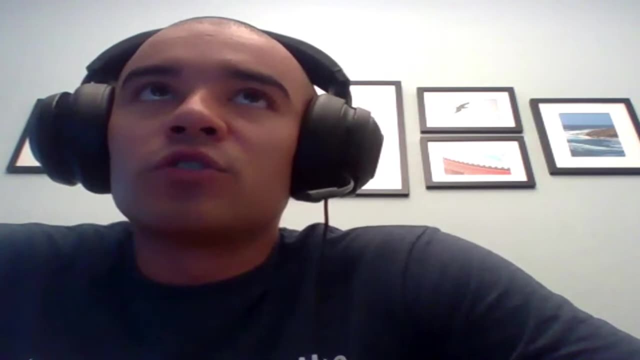 freshwater clams. You could- I mean you could always. you could eat anything once but the. the main issue, at least here, is that there's water quality issues, so you don't want to consume animals that are in. you know, most of our freshwaters aren't exactly the most pristine, but the short answer is in a lot of. Asian countries. the Asian clam is a food source, just like it is elsewhere, and to to add to that, Asian clams do only live a couple years, so in terms of bioaccumulation or other issues, it's less of a concern. A freshwater mussel lives a lot longer, so if you ate one of those, you're. 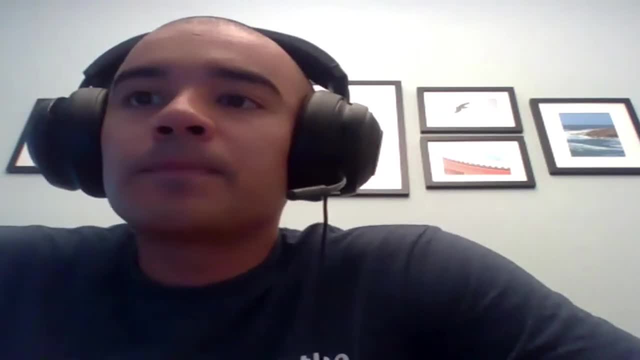 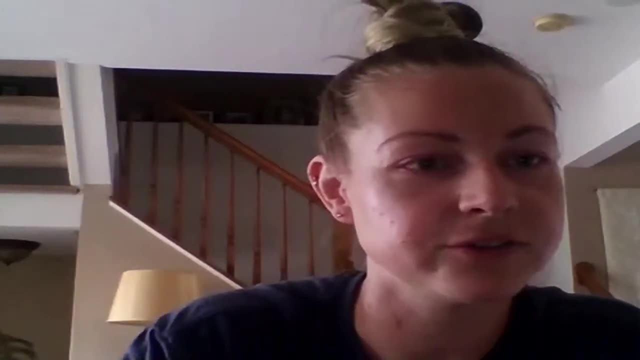 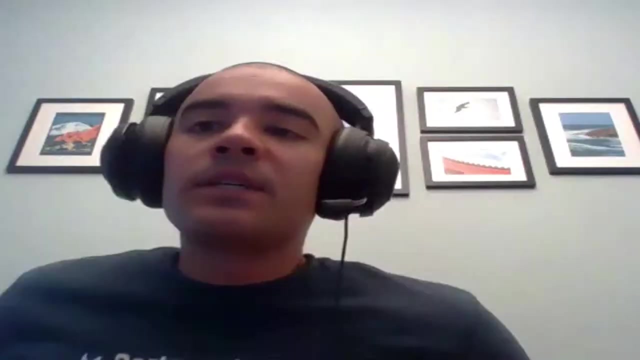 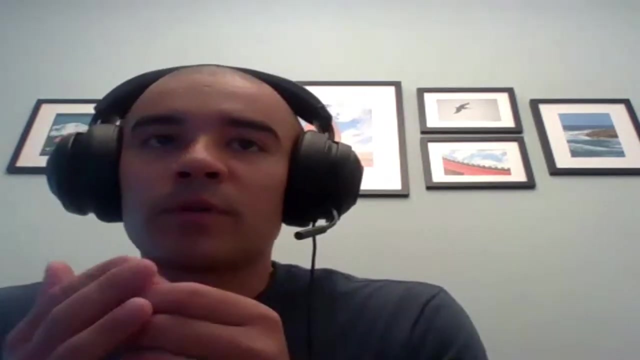 probably eating 20 years worth of pollution. Great thanks. So another one was: how do you tell the difference between the fingernail clam and the Asian clam? Yeah, that's actually pretty easy. so if you have a small clam in freshwater, you know it's one of those. if you rub your rub your finger over the shell, an Asian clam is always going to. 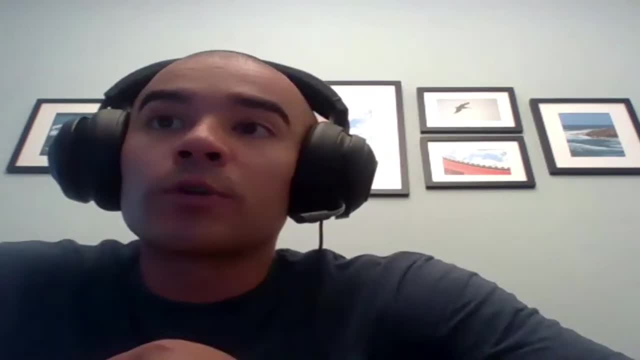 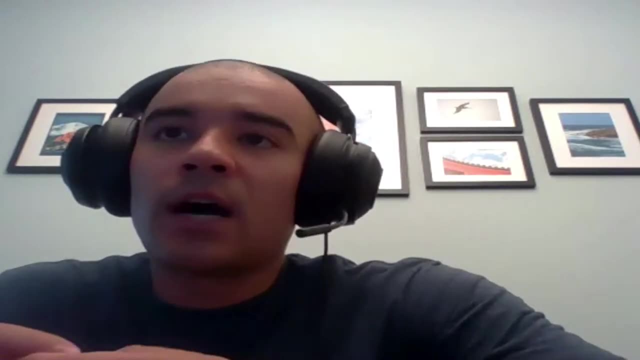 have really rough ridges. You're going to be able to just like a quarter. you're going to be able to put your fingernail or something like hard like that, and you'll feel each ridge kind of like the cog of a wheel. Fingernail clams will be smooth. 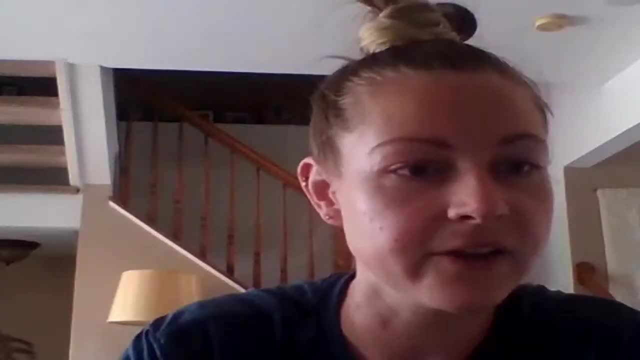 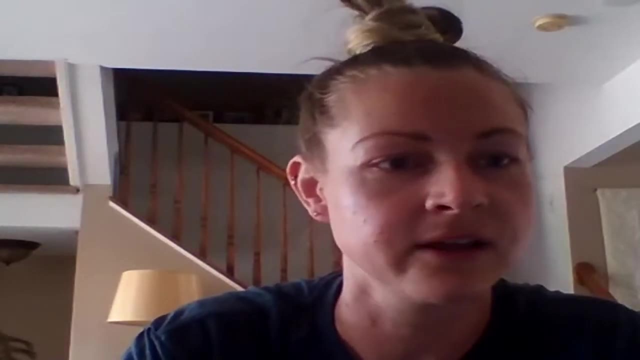 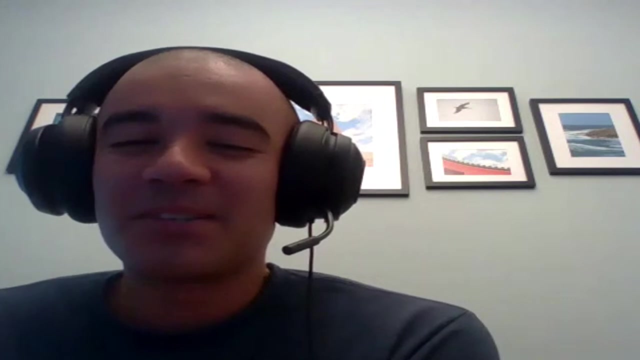 All right, another question that came in. it might some further information about the zebra mussel. it might be more of a taxonomy question, actually it's: why is the zebra mussel not considered a mussel? what's, what is the actual distinction? Yeah, so that's a good question. My quick answer and it: 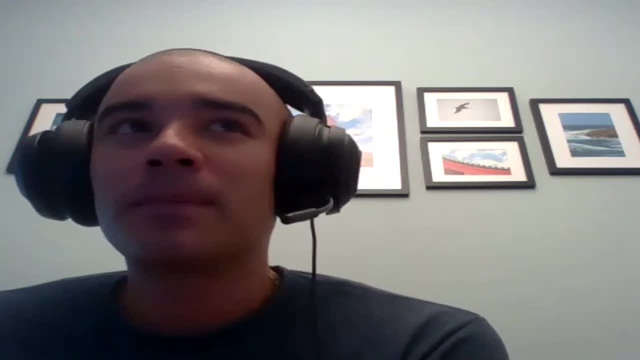 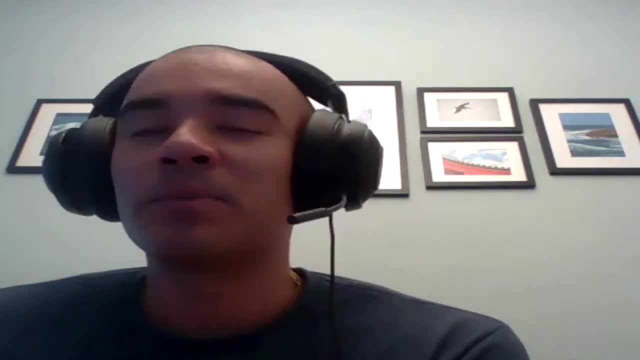 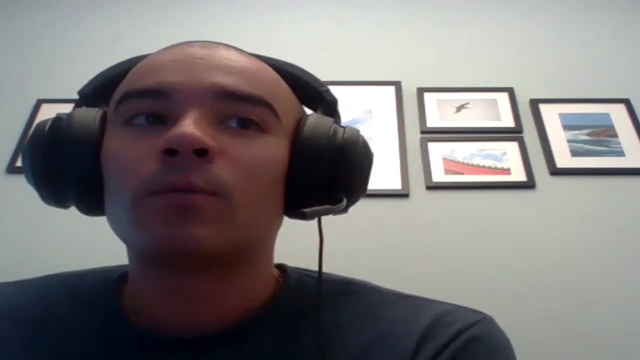 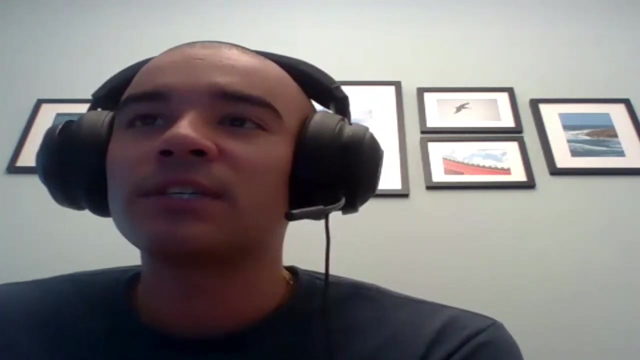 I mean, you know, scientists usually don't use the common name because it confuses people and common names aren't standardized or anything. So, case in point: there's some researchers that call what I call freshwater mussels freshwater clams. So really the clam versus mussel terminology is kind 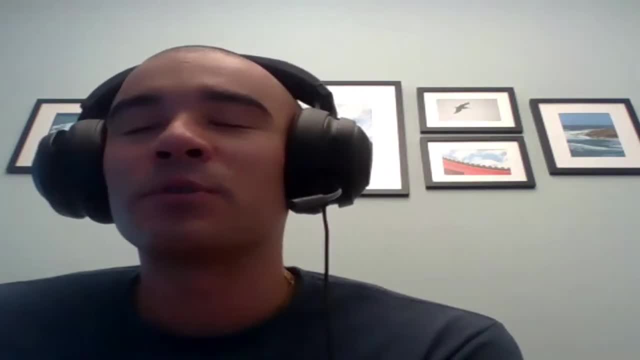 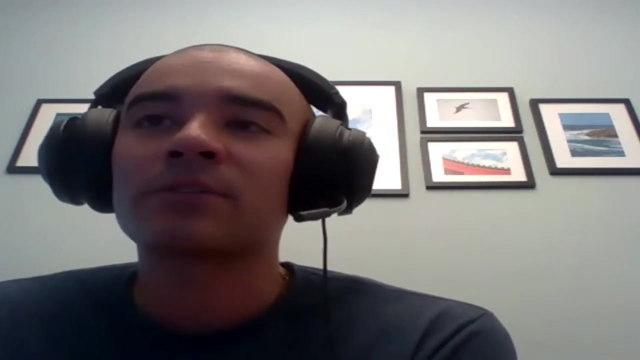 of a sloppy one that it's really. you know there's, I'm sure there's some kind of history with seafood and everything. but you know, if you talk about a true I guess mussel, the mussels, that those tend to be the epiphanal bivalve. So those are things that actually attach to things, Things. 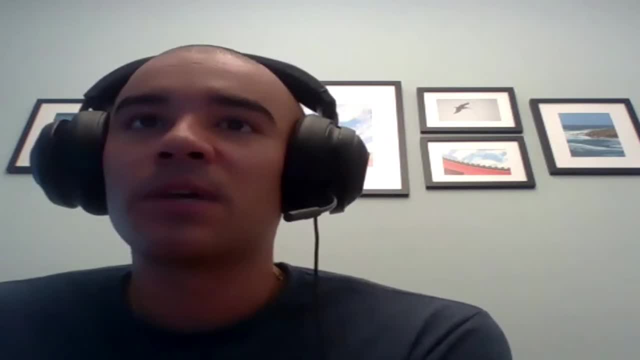 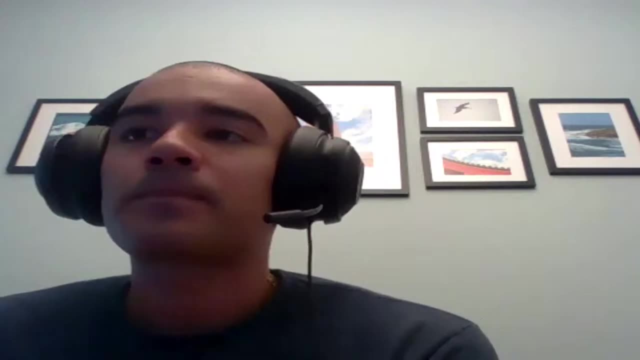 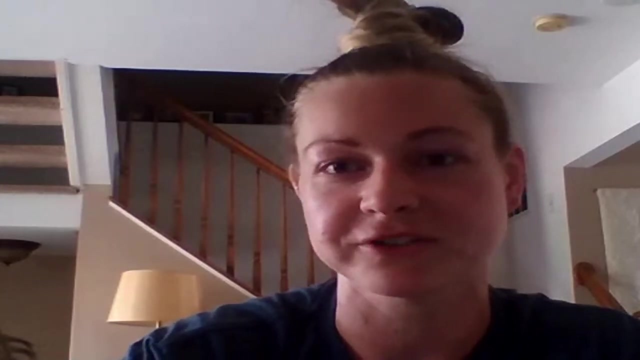 like blue mussels, zebra mussels, rib mussels. They provide, or they produce bissell threads that attach physically to structures. All right, great, I think we'll do maybe just two more. and then again, folks, if you had any burning questions for Kurt, please send them to him via email. But how about? why don't we eat freshwater mussels? Yeah, so basically you know for one, I guess I'll touch upon it. Freshwater mussels are protected in a lot of states, so you you don't really want to just touch them or harvest them. We have special permits, scientific collection permits, for all. of our states that we work in. Additionally, they're long-lived species and they live in, oftentimes, waters less than pristine, so you don't want to get sick. They also harbor a couple freshwater parasites as opposed to saltwater. Saltwater tends to be a lot more clean in general. 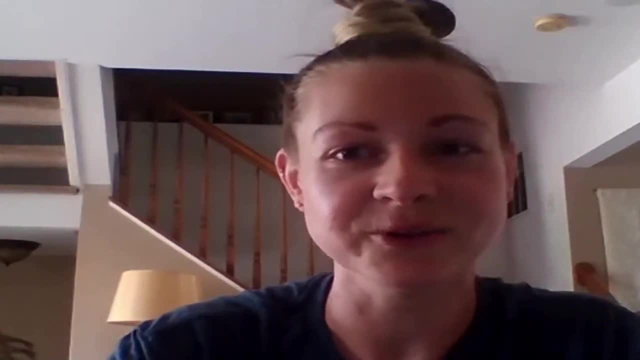 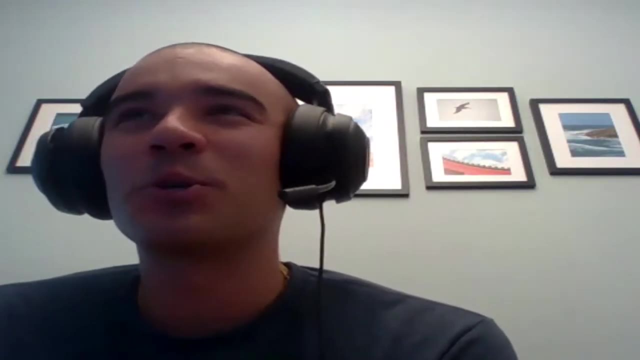 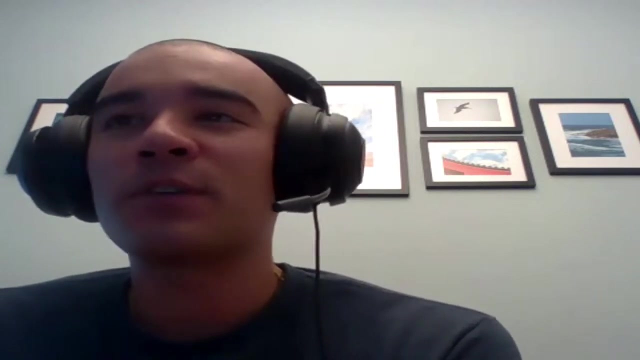 All right, we'll do one more. I think this is a good one. How did you get into freshwater mussels? Great question. So I guess long story short would be. I went to school and wanted to study something aquatic, Perhaps fish, and then I kind of got into the oyster world. So initially I worked for the Rutgers Haskins shellfish research lab and then I kind of moved my way into the Delaware estuary over to partnership for the Delaware estuary And we didn't do so much with oysters but we did a lot with freshwater mussels. So we we do support shellfish research. 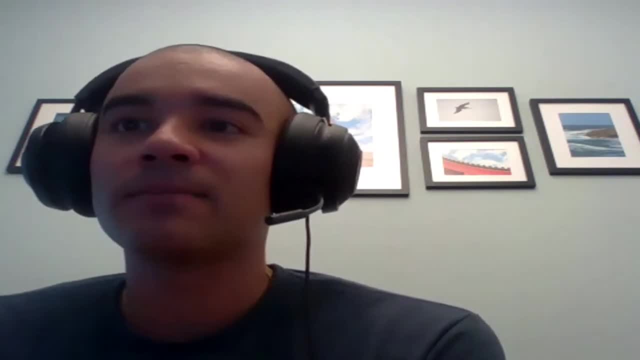 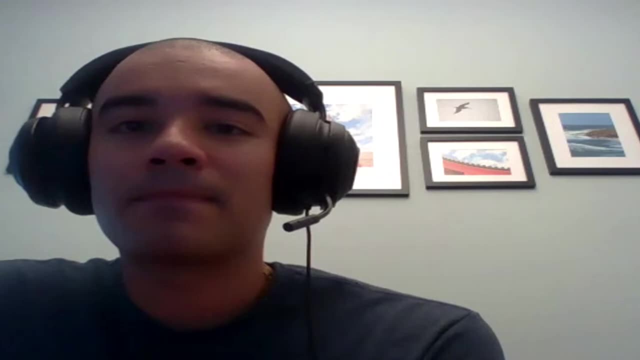 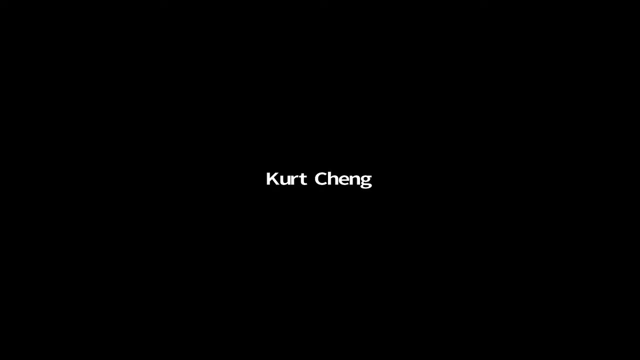 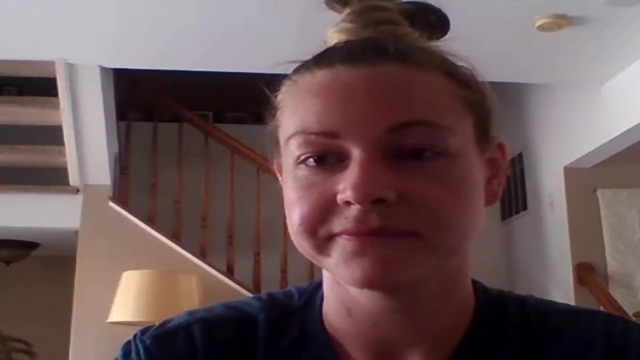 in general, but freshwater mussels kind of grew on me, I guess. Great thanks, Kurt. Yep, no problem, Thanks guys. All right, I think we're going to turn it over to our next speaker today for this session. Matt, If you're ready to pull up your presentation, we'll move on. 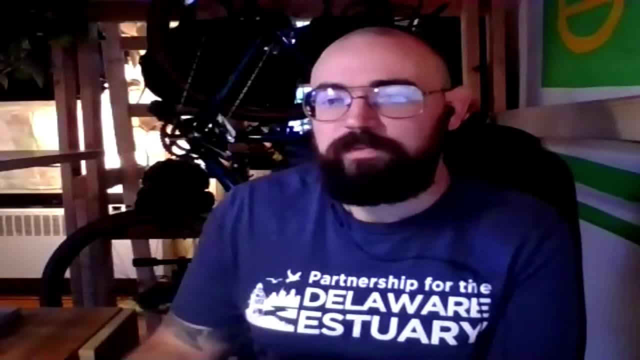 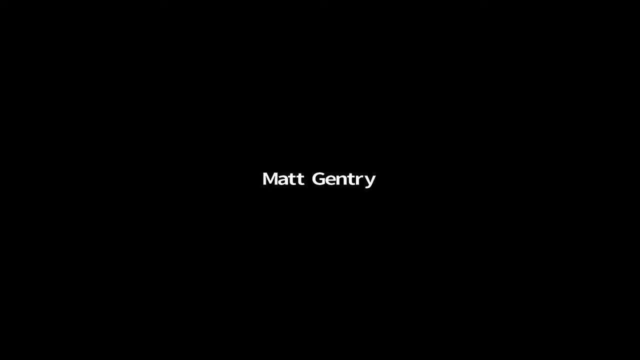 Yep, hi everyone. I'll be getting my presentation up in a moment. Thank you, Matt, for the introduction and thank you for your amount of位ting. And so, Matt, I'll be parameter spacing and I'm setting up a lifetime. So, Matt, those of you if you do want to, let you get in here, but we may not be able to show that. 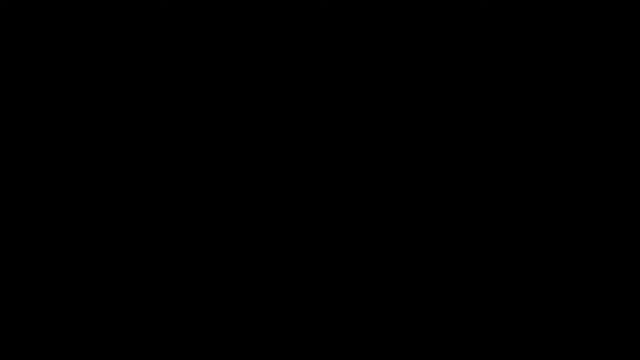 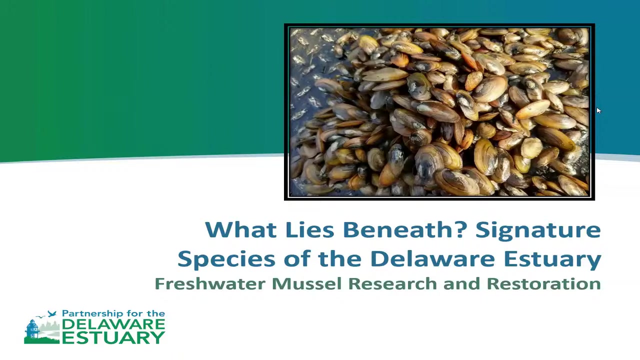 All right, All right, is everyone able to see that? Yep, you're good, Matt, Alright, great. uh, thanks for the introduction. uh, good afternoon everyone, and thanks for tuning in. My name is Matt Gentry, about 칠, regrets your time without me. we are so grateful to have you to step right in with the time. sorry, ever after the event we've had, but we will try and perfect the presentation. but do remember if, Virginia, you have to stay until Pew BILL. Thanks for the good and the best. 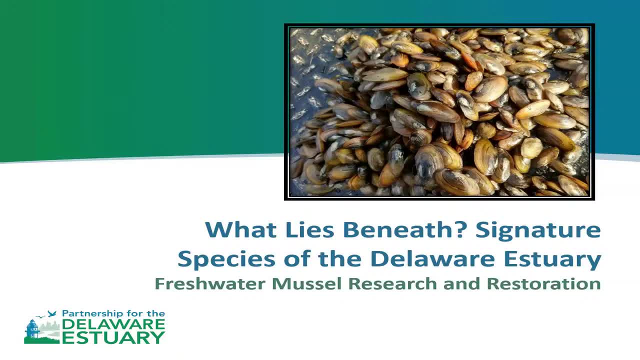 and I'm a shellfish specialist at PDE. I've been with PDE for a little over two years and most of my time has been focused on work relating to freshwater mussel recovery and restoration, and I also design and fabricate equipment that we use in the field and lab for various projects. 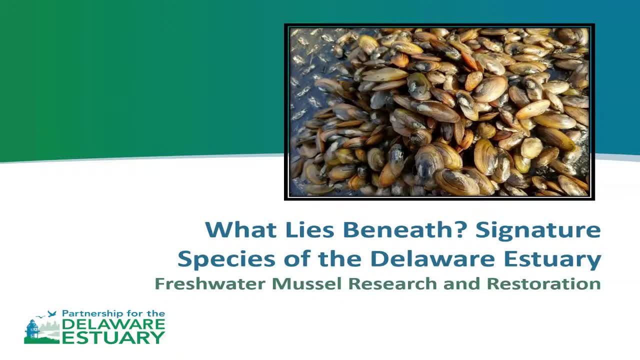 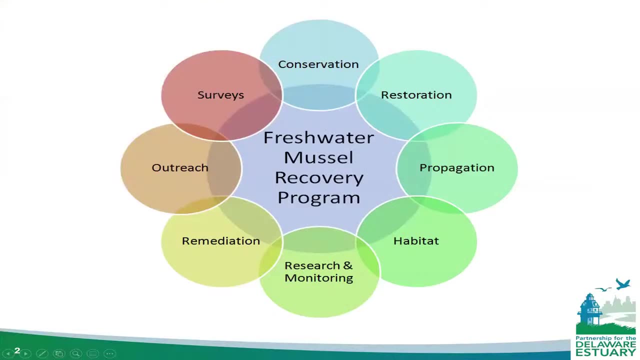 This portion of the webinar will focus on some of the research and restoration work that PDE does with freshwater mussels, and if you have any questions during the presentation, please follow the same procedure as the last one with the Q&A feature: The freshwater mussel recovery program. 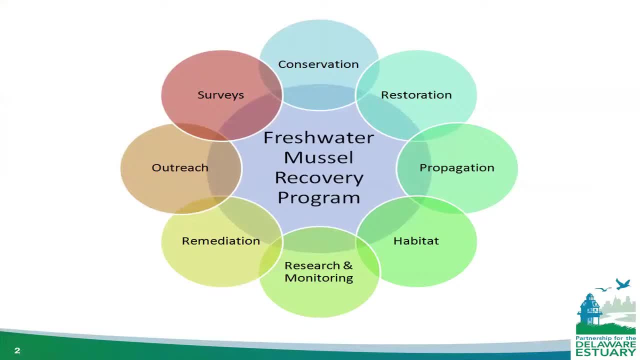 or FMRP, is a comprehensive program intended to support the health of our region's freshwater mussel populations. It's part of a basin-wide shellfish strategy, which we also have. that includes species such as oysters and rib mussels, and there are eight primary facets to the FMRP. 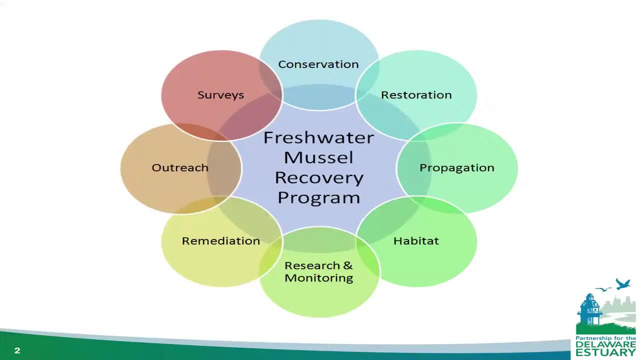 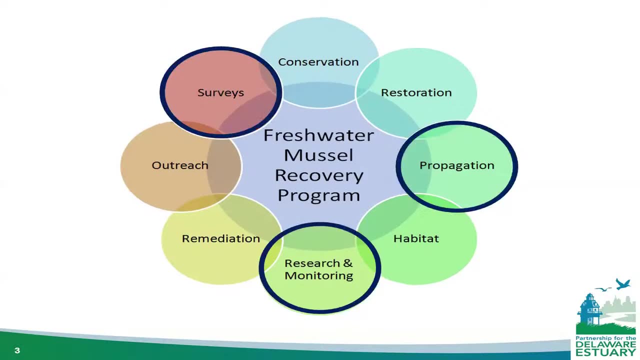 which you can see here as conservation, restoration, propagation, habitat research and monitoring, remediation, outreach and surveys. Although PDE is involved in all aspects of the FMRP, today I'll be discussing some of our efforts relating to the three circles here: surveys, research and monitoring and propagation. The first 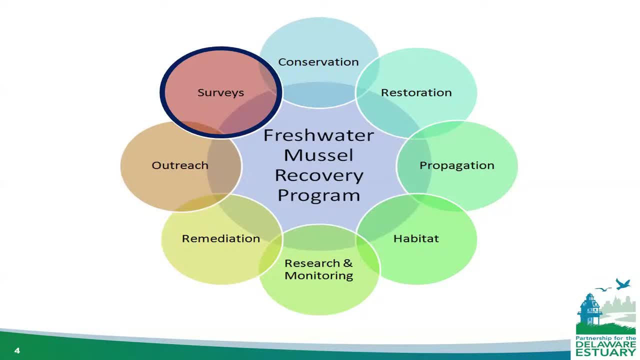 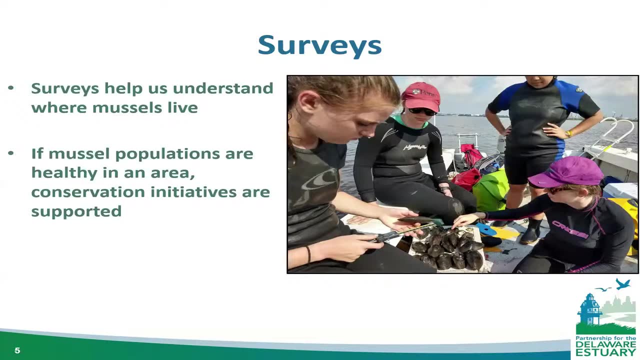 facet I'll be discussing is the use of surveys and how they fit into the conservation of freshwater mussel populations. By learning where mussels currently live, we are better able to understand the conditions that enable healthy mussel populations. Some of these conditions are the physical and chemical characteristics of the water body known broadly. 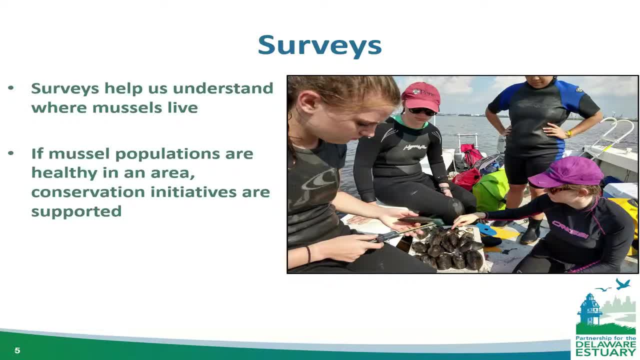 as water quality, and others are the characteristics of the substrate, such as the sediment grain size and the stability. for example, if a stream is very flashy and will lose a lot of sediment, Many people are surprised to learn that there are some very healthy mussel beds in our region. 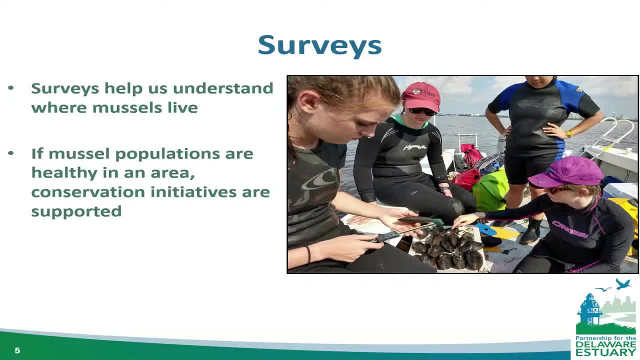 including right near Philadelphia and Camden, on the Delaware River. These beds are functioning without outside help, So the best thing we can do for them is to continue to support efforts that improve water quality and habitat, and those would be the conservation efforts of the FMRP. 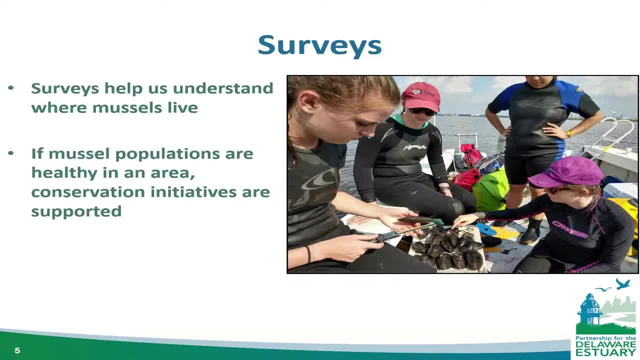 This photo right here is of a snorkel survey that was conducted to help assess the conservation status of one of the mussels that Kurt was talking about- the tidewater musket, and this was a survey in collaboration with the Academy of Natural Sciences of Drexel University. 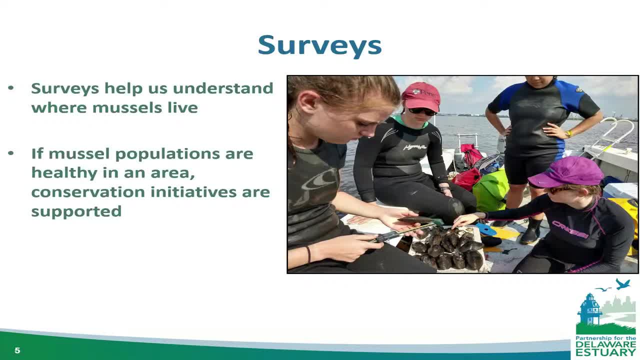 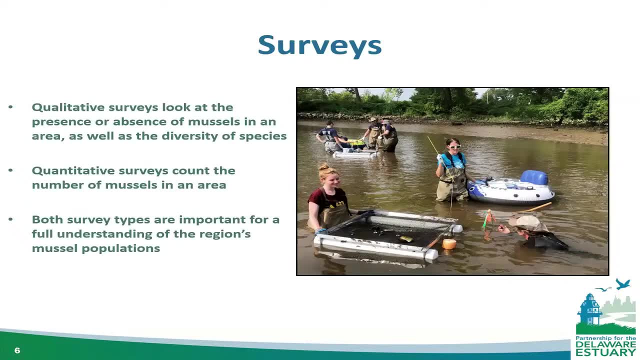 the Pennsylvania Natural Heritage Program and the Western Pennsylvania Conservancy. There are two broad categories of surveys that we conduct: qualitative and quantitative. The qualitative surveys are just looking to see if mussels are there and if they are there, what species are there, what kind of diversity we have Quantitative surveys on 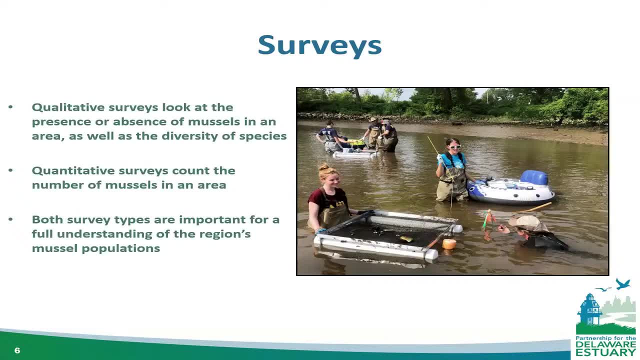 the other hand, actually count the number of mussels in a specific area. These surveys record size classes, which can help us understand the population trends, for example, if there's only adult mussels there or if there's a healthy bed with reproduction and a lot of different species. 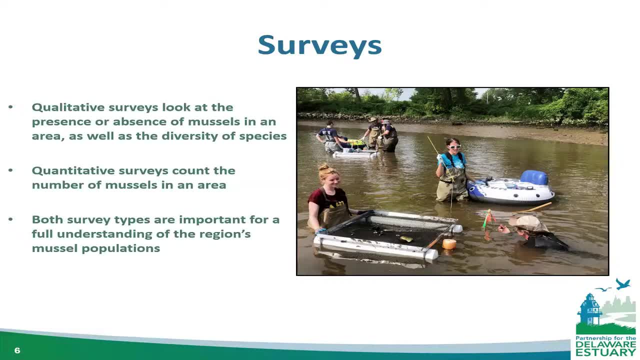 PDE has conducted surveys in more than 75 bodies of water in this region, and both survey types are essential so that we can understand fully how the region's mussel populations are doing. This photo is from a quantitative survey that we did right by. 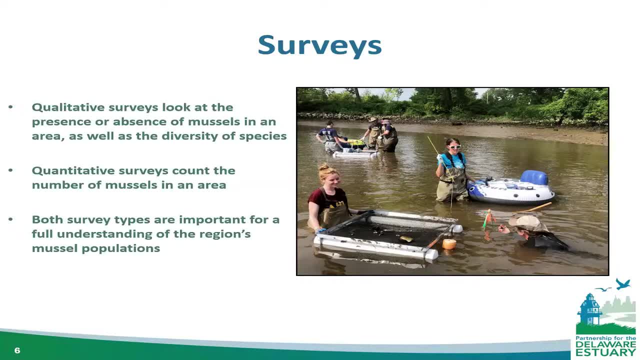 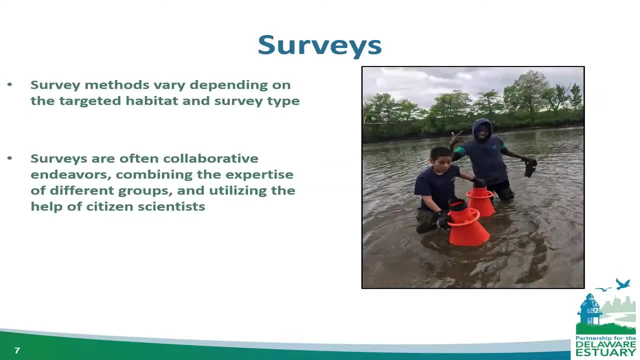 Bartram's Garden in southwest Philadelphia last summer. in summer 2019, on the Schuylkill River. Some of the survey methods that are used to assess freshwater mussels involve snorkeling, wading and even side-scan sonar. Different methods will be used depending on the environment. 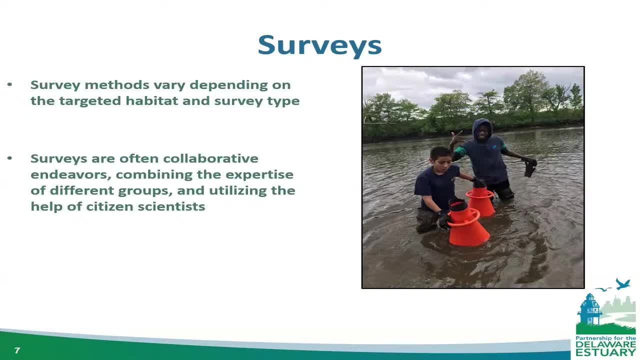 that we're surveying in, And surveys are often collaborative efforts combining different groups' expertise and also using citizen scientists and school groups. So this photo here sort of shows the outreach component of the FMRP that ties into surveys. These were some students from Camden, New. 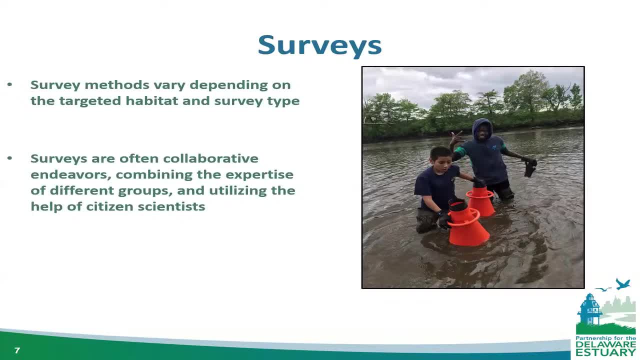 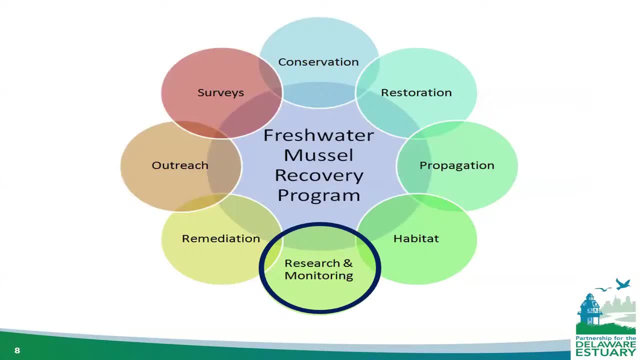 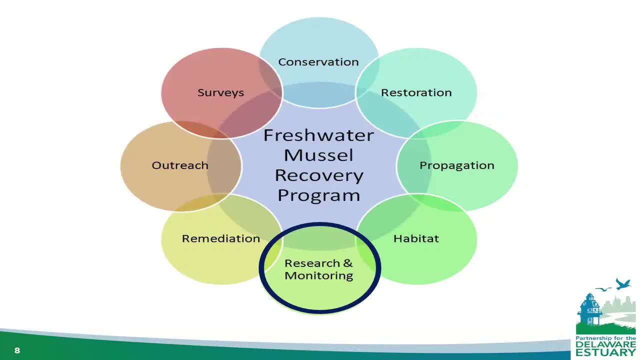 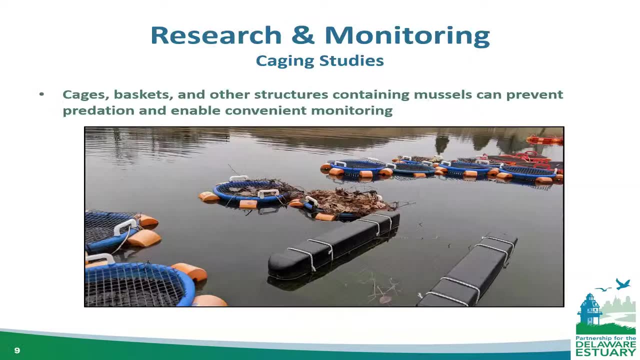 This work advances the scientific understanding of everything, from which host fish mussels use to the mussels' ability to survive in different environments. The most common method of field research and monitoring that we do is the use of cages to grow mussels in natural water bodies. 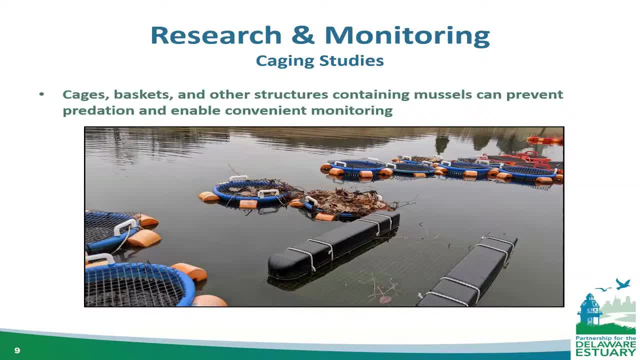 Here you can see some floating baskets that we built based off of designs from other groups, that we've made some improvements on, as well as larger floating cages that are traditionally used in oyster aquaculture, and all of these contain mussels. Keeping the mussels in cages. 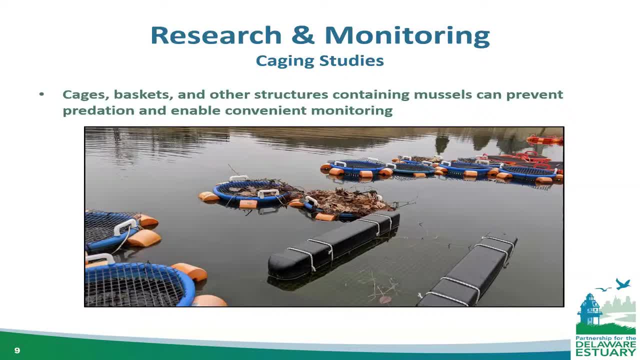 can protect them from predators such as muskrat, raccoons, large fish and birds, and also allows us to easily monitor the growth of these mussels. We used floating cages like those seen here, as well as benthic cages that would be anchored to the bottom of a stream or a river. 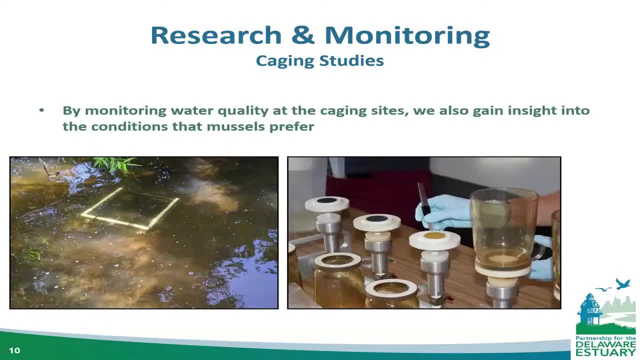 Along with monitoring mussel growth and survival, we monitor the water quality at our study sites. This includes dissolved water quality, such as pH, temperature, dissolved oxygen and salinity, but it also includes measuring the particulate matter floating in the water, which is what the 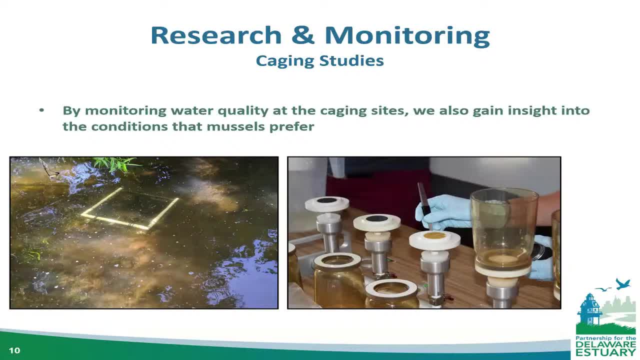 mussels eat as food. On the left here you can see one of our cages anchored to a stream. bottom and on the right is a vacuum filtration setup that we use to filter out particles from the water and analyze their composition. We look for things such as the organic content in the 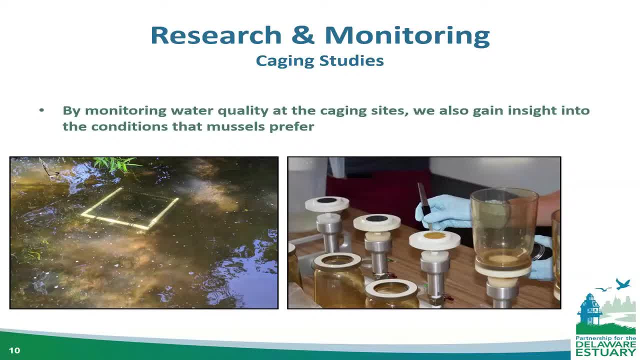 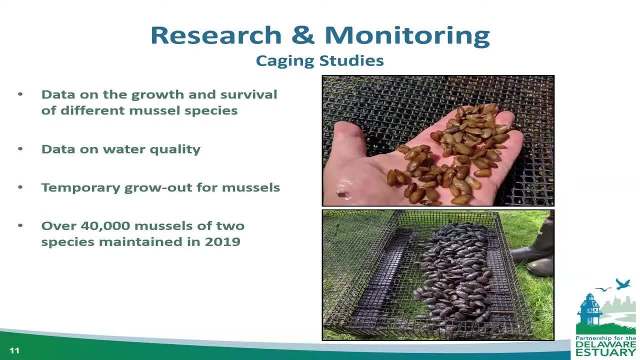 water, because that's ultimately what the mussels will be transforming into nutrition. Water quality varies between locations and throughout the year, so by monitoring it along with mussel growth, we can gain some more insight into what conditions the mussels prefer. Caging studies that we conduct give us data on growth and survival. 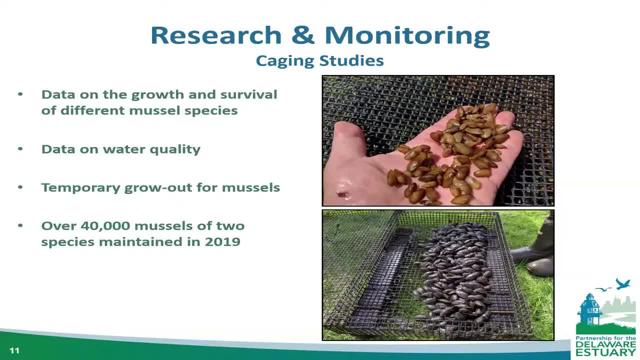 rates of different species, information about water quality and allow us to temporarily store mussels that will be used in future restoration work. We work in ponds maintained by partners such as Winterthur Museum and Gardens, Longwood Gardens, Suez and various state and. 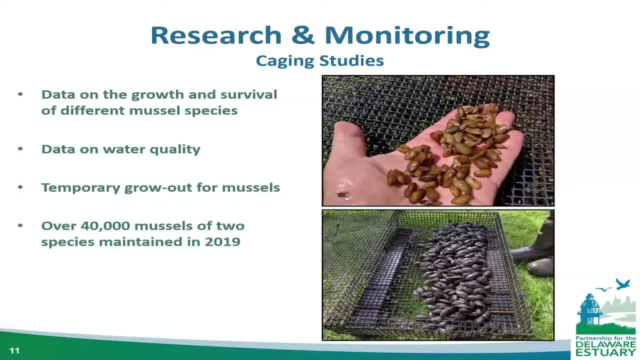 local governments, among others, to test varied conditions and assess restoration potential. By monitoring these mussels and the water they live in, we also learn about their ability to extract nutrients from the water column and can estimate their potential use for remediation of nutrient-rich waters. In 2019, we maintained over 40,000 alewife floaters in eastern pond mussels. 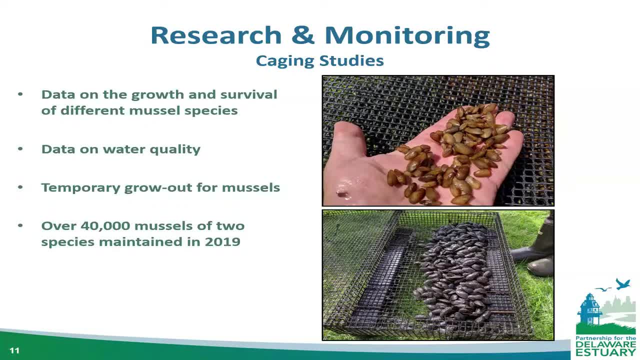 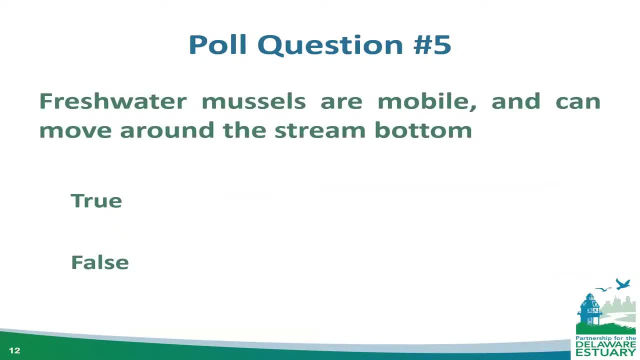 and these photos show mussels that are two months old at the top and about two years old at the bottom photo. Before we move on, I've got a poll question. so, Leah, if you could please bring up that poll- True or false? freshwater mussels are mobile and can move around the stream bottom. 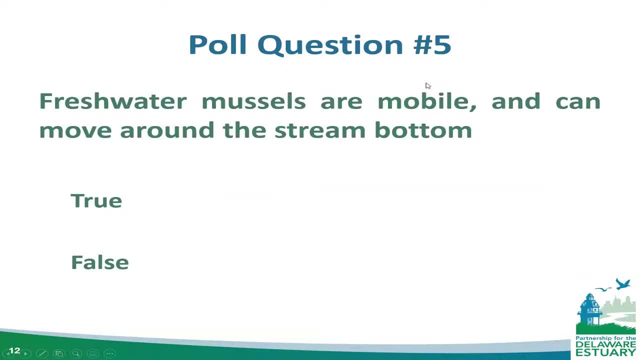 All right, yep, the majority of people got that correct. It's true, A mussel can burrow and move around at will. They can't move very far, but they can move sometimes upwards of a meter per day, especially in tidal areas. 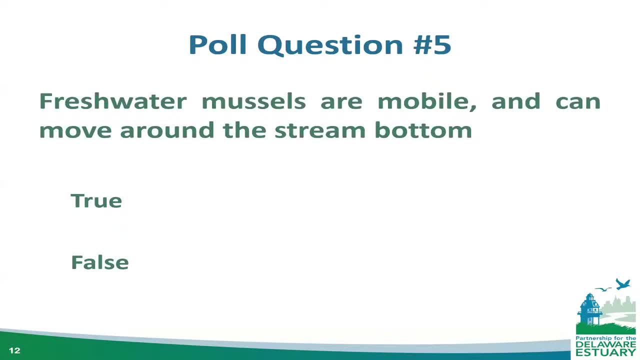 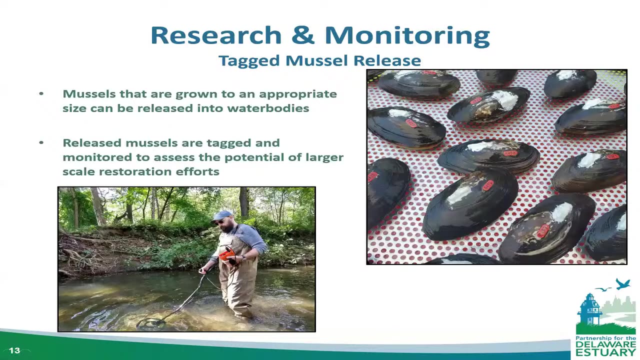 They can move up depending on where the water level is, and they can find more suitable substrate to anchor themselves in using their foot. Tagging and releasing mussels can provide many of the same data as cage mussel studies. Doing this on a regular basis allows the mussels to freely move around and we are able to assess their growth in. 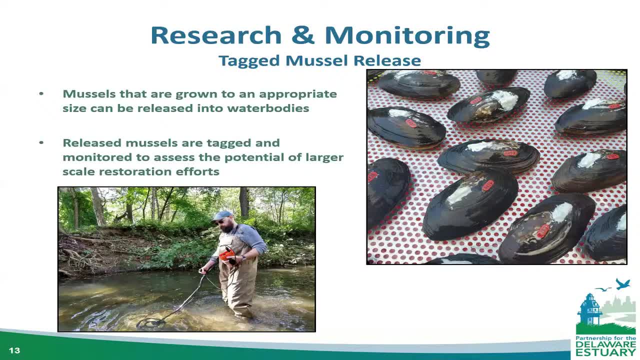 an environment that is more natural than a cage. This includes gaining some insight that we don't get from cages, such as predation. If we find broken shells when we monitor these sites, we're often able to determine what type of animals ate the mussel based on the damage done to the shell. 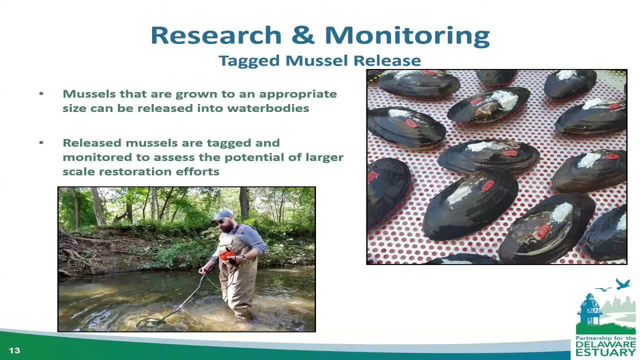 The white marks on the mussel shown on the right are electronic pit tags that are applied with marine epoxy that we can scan for using the device in the other photo. This doesn't hurt the mussel. Finding these tagged mussels helps us learn if they stay in place where we released them. 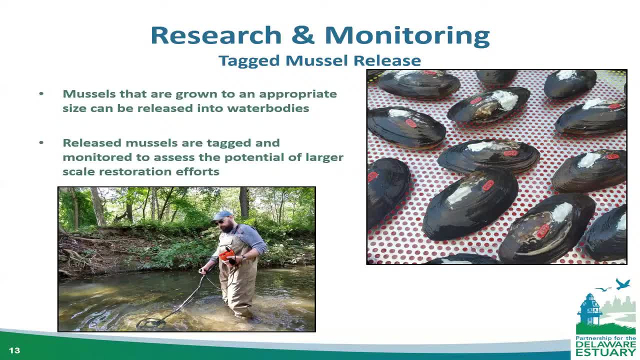 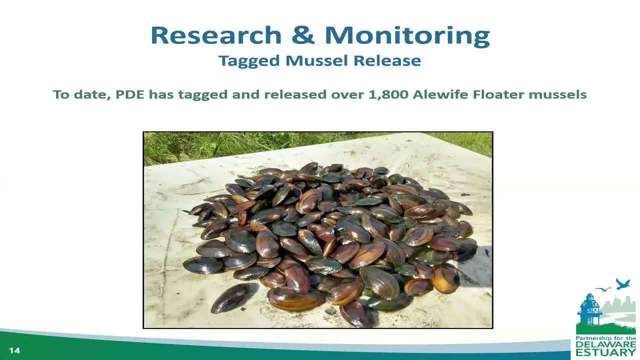 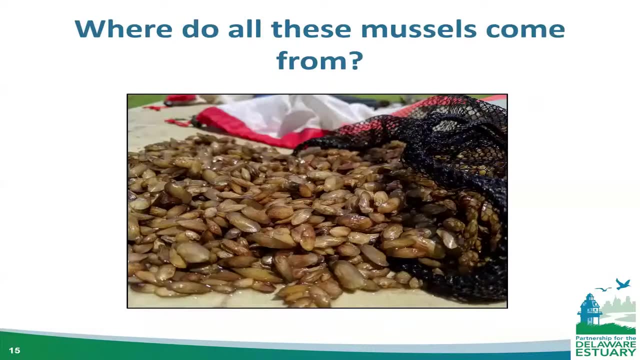 or if they moved around to more suitable habitat and if they stayed in place, then that stream could be a potential future restoration site. To date, we've tagged and released over 1,800 alewife floater mussels. So where do all these mussels come from? In areas with abundant natural mussel beds. 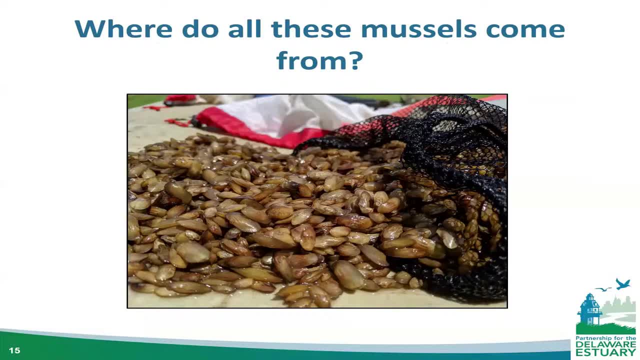 animals can be translocated to either a establish a new bed or supplement an existing, more sparse bed. Because there are not abundant mussel populations in our region, we rely on a method that is common in other groups of organisms, such as fishes. the final FMRP component that I'll be discussing: Propagation. 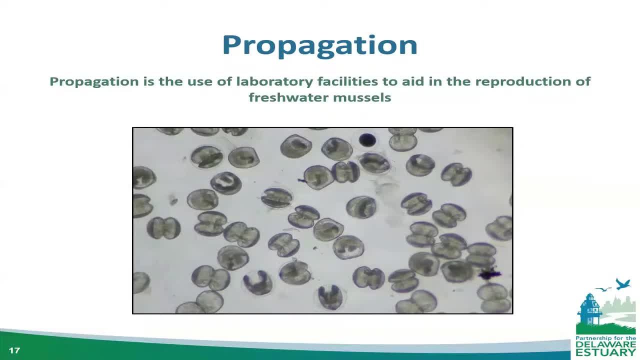 Propagation is the use of a hatchery or a laboratory to help spawn and grow mussels. This photo shows the mussel larvae, or glochidia that Kurt was talking about earlier, that have been extracted from a adult female mussel. They have that Pac-Man-type shape that they use to clamp down on the fish gills. 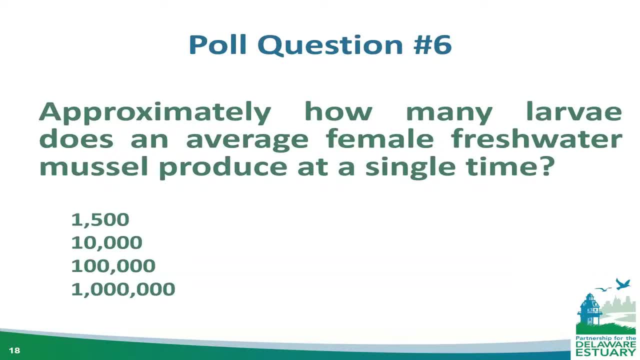 Before I continue we have one last poll question. so, Lee, if you could please bring that up Approximately, how many larvae does an average female freshwater mussel produce at a single time? 1,500,, 10,000,, 100,000, or 1 million? 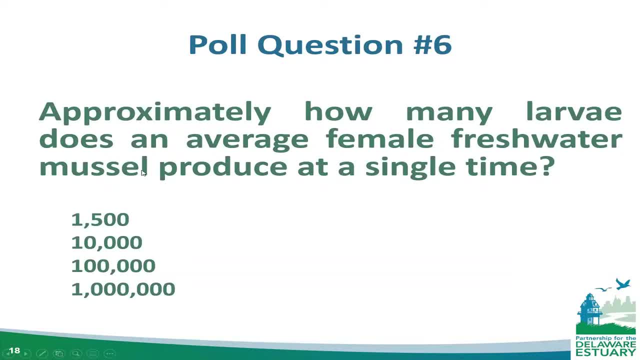 All right, Yeah, it looks like most people said either 10,000 or 100,000.. So the answer to that is: those are correct. The answer depends on the species and the size of the mussel. The mussels that we usually work with in the lab generally have between 60,000 and 200,000 viable larvae. 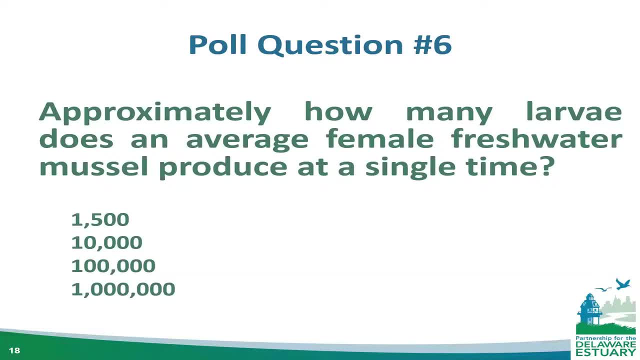 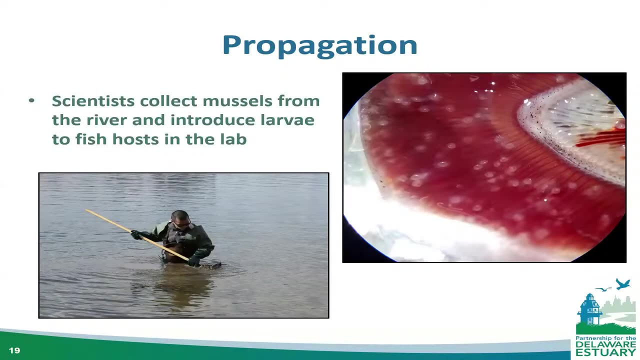 but there are some species that are closer to producing around 10,000.. And some species may also have multiple broods of larvae per year. Here we can see Kurt on the left who presented before me, collecting some freshwater mussels To get them into the hatchery for propagation. we go out with waders and clam rakes. 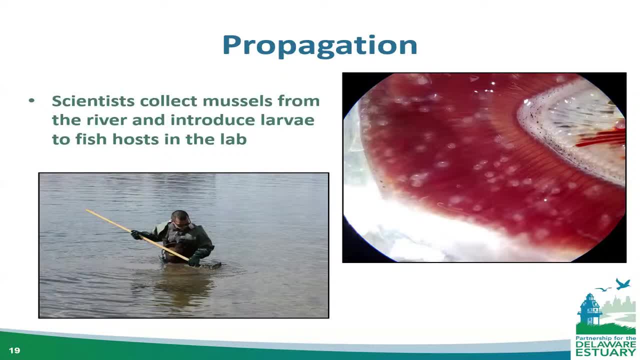 and dig up from a natural, healthy mussel bed that we know has abundant animals in it. And on the right is a close-up photo of a fish gill that is infested with the mussel glochidia. Generally, this doesn't do great harm to the fish. 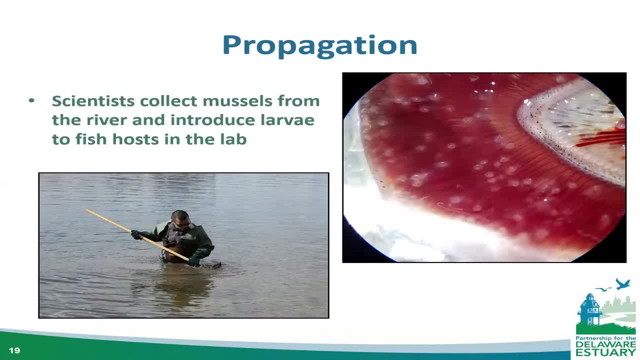 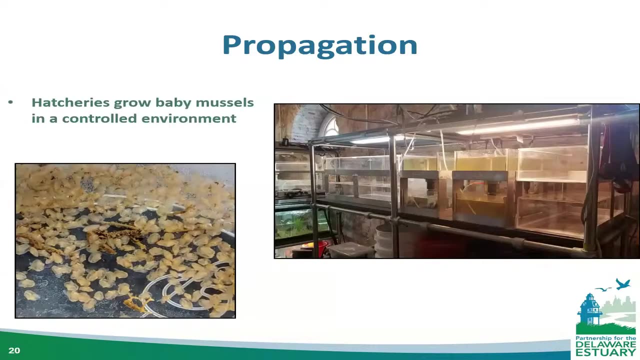 Since it's in a controlled lab environment, we can kind of control how many larvae are going to latch onto the fish gills to make sure they don't get suffocated, And after the propagation occurs, the fish and mussels are both released back into their native water bodies. 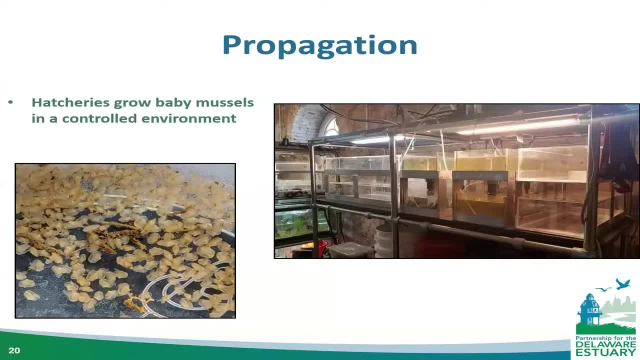 Hatcheries allow us to grow baby mussels in an environment where we can control the water quality and other variables. New equipment, diets and systems are designed and tested constantly. The photo on the left is of some juvenile mussels that are a few weeks old in a petri dish. 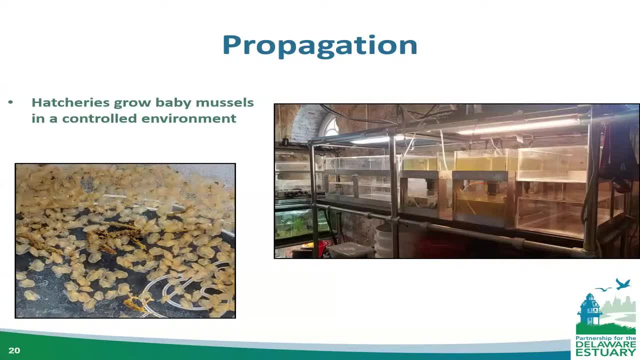 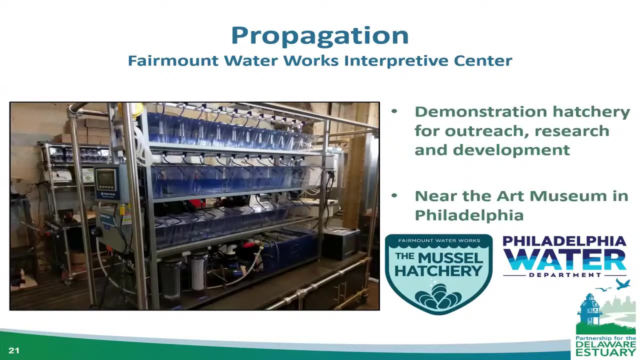 And they're about one millimeter in length. On the right are some of the recirculating aquaculture systems that we designed and built for growing juvenile mussels in the hatchery. The hatchery where we do our propagation work currently is at the Fairmount Water Works Interpretive Center. 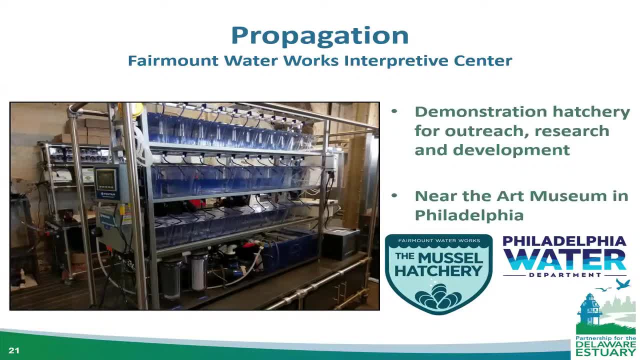 This hatchery was built in 2017 and is located along the Schuylkill River and owned and operated by the Philadelphia Water Department. In close proximity, it is the largest water supply plant in the United States. We've been working with the National Association of Aquaculture Scientists for research and development. 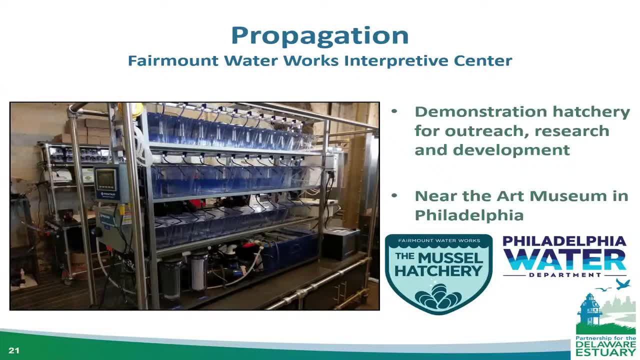 to create a grant to support this collaboration with our scientists at PDE. We've been developing new techniques for mussel propagation here, such as experimenting with different diets and aquaculture systems for growing the juveniles. We also conduct experiments here to discover which fish species may be viable hosts for different mussel species. 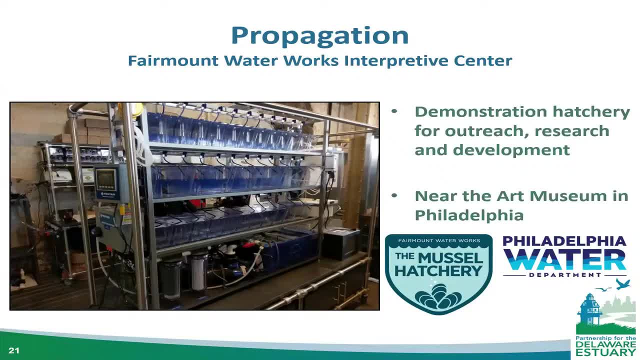 This facility is normally open to public viewing, with its primary goal being outreach, but is currently closed due to the pandemic. Because of its broad uses, this hatchery fits not only into the propagation process, but also into the water supply system goals of the fmrp, but also into the outreach and research goals and for 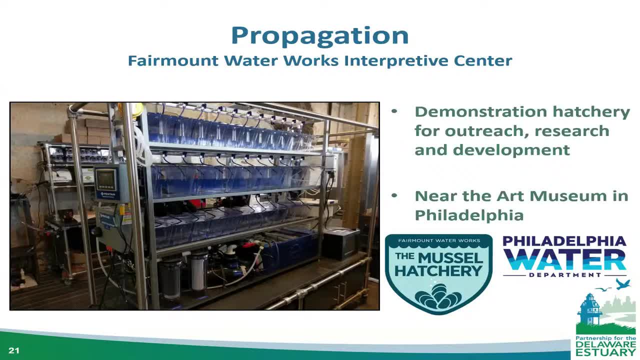 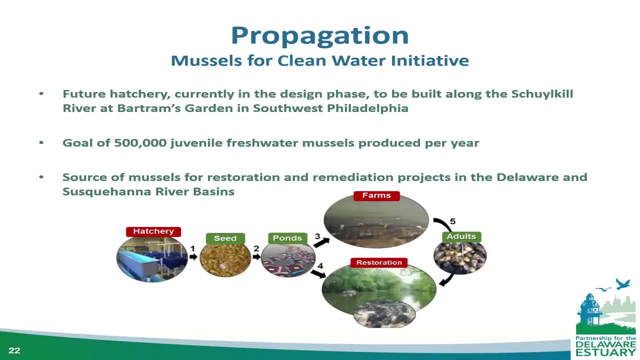 anyone that doesn't know or isn't familiar with Philadelphia. this is right near the art museum along the Schuylkill River. and finally, I want to touch on the mussels for clean water initiative. it's the next big step for PDE. we're currently in the process of designing and building a production scale. 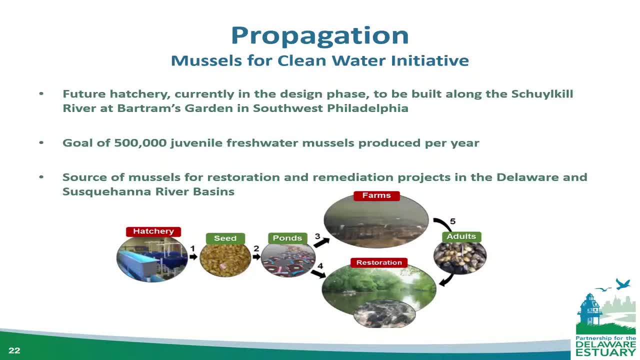 freshwater mussel hatchery on the banks of the Schuylkill River at Bartram's garden. this hatchery will produce up to 500,000 juvenile freshwater mussels every year for use in restoration and remediation projects in the Delaware River Basin and also in the Susquehanna. this will be the first freshwater mussel. 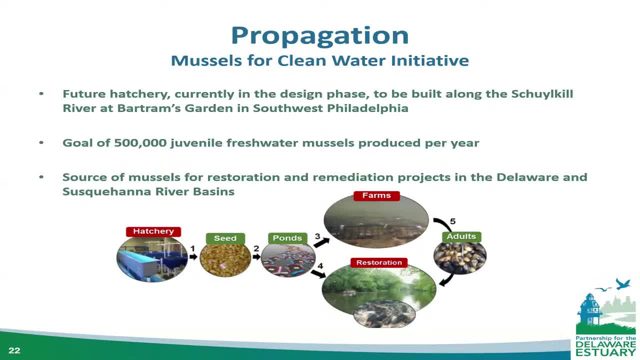 hatchery built for the explicit goal of improving the health of the water that we all rely on, and it's slated to begin operation in 2023. thank you so much for tuning into this webinar. I hope you found it interesting and have a better understanding of the nature of freshwater mussel hatchery and the 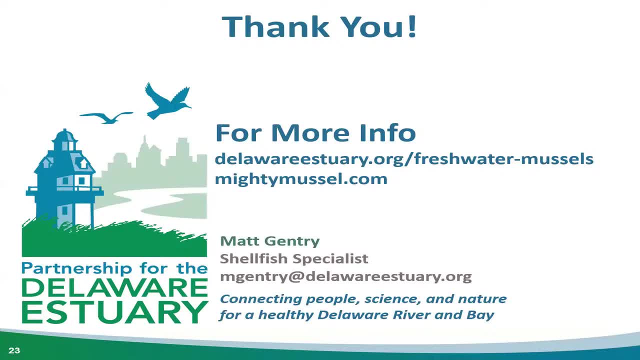 understanding now of some of the things that partnership for the Delaware estuary is doing to improve the status of freshwater mussels in our region. if you'd like to know some more information about mussels, please visit the sites I've listed here: mightymusselcom and our website has. 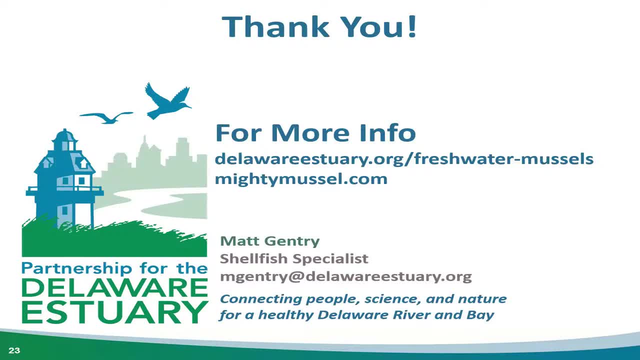 some information about freshwater mussels, among other things, and feel free to send me an email at mgentry at Delaware estuary org. if there's any questions you have. that I'm not able to answer today, so I think we have a few minutes for questions now if, Emily, you want to those. 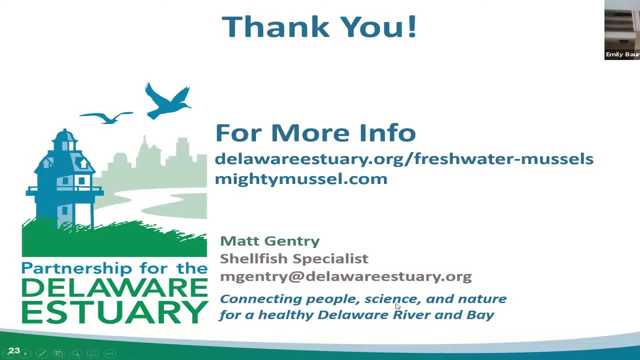 up, all right. yeah, thank you very much, Matt. that was great. I'm just gonna go ahead and put your email address in the chat as well, for any of the questions that we don't get to. you can maybe ask you one or two. here's one does keeping. mussels in cages prevent them from attracting fish hosts for reproduction? yeah, so a good question. when they're in cages, they're generally juveniles that aren't able to reproduce yet. we have found that with some of our mussels in those cages or in other systems, they are fertilizing each other, but that doesn't. 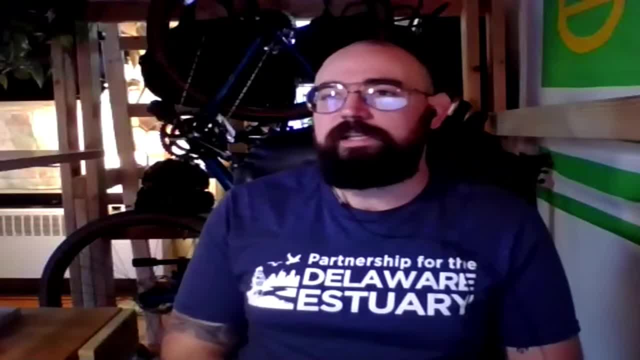 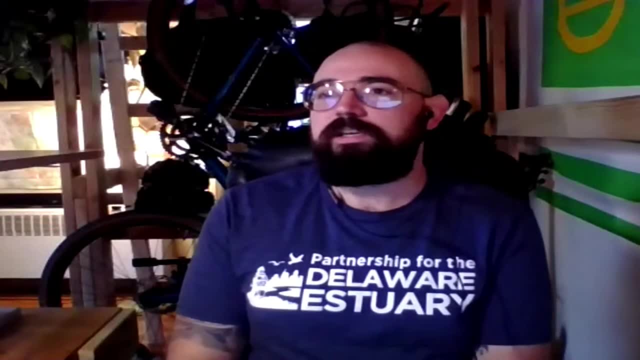 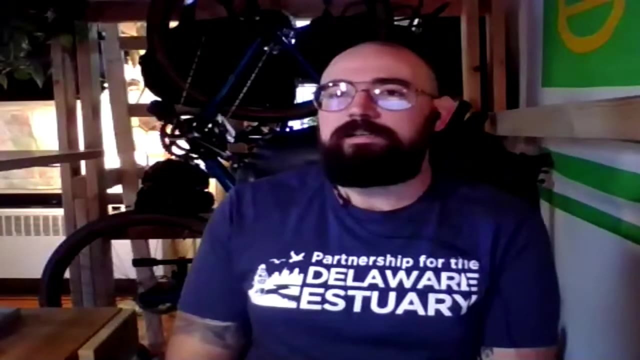 really happen until at least two years of age and generally at that point we're using them for other projects. so the vast majority of our mussels that we have in cages are going to be smaller juveniles that aren't really have a reproductive size or age. the pacific artists use for such purposes plates and sujet. 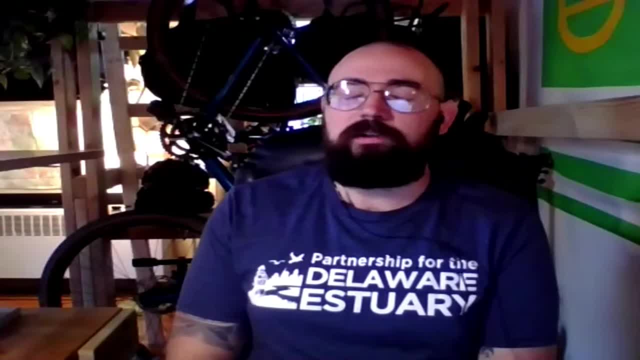 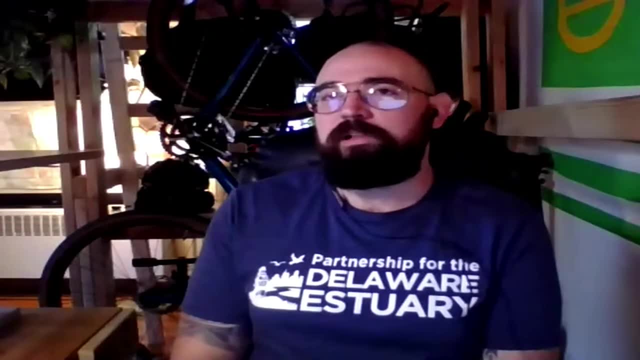 and we do the cages some of them, if we have larger mussels in them, the mesh size or the size of the cage is large enough that we do have fish, smaller fish, kind of going in and out of the cages because it's good habitat for them as well, great. next question: how long do freshwater mussels typically live? that depends on the species. like with most things, with freshwater mussels it's a very large and diverse group, but some species in our area can live up to around a hundred years- great. here's another question, Matt. this is more I. 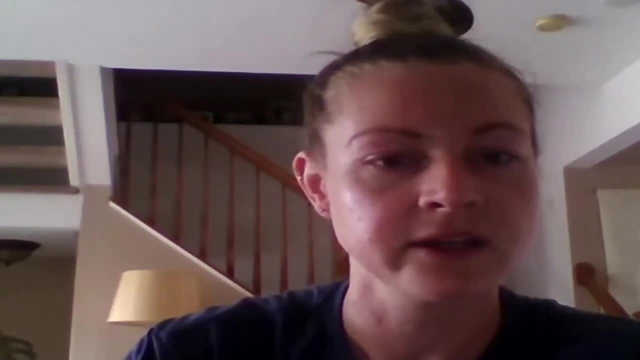 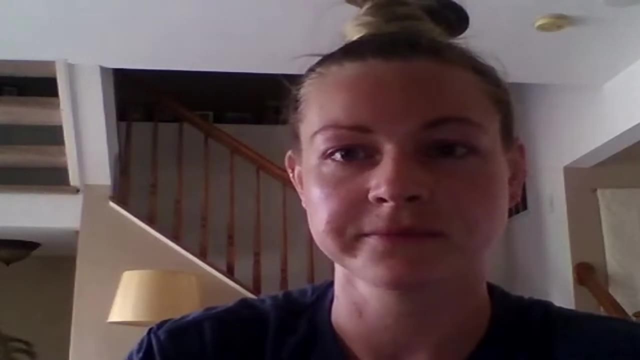 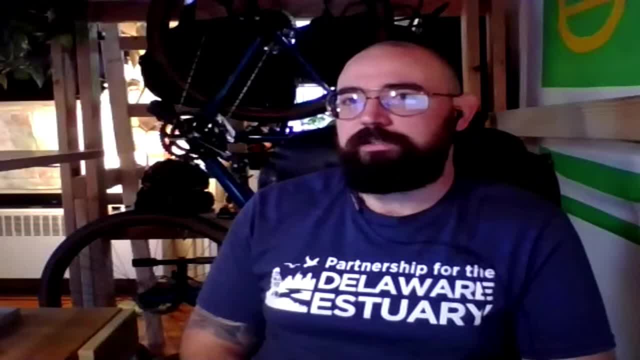 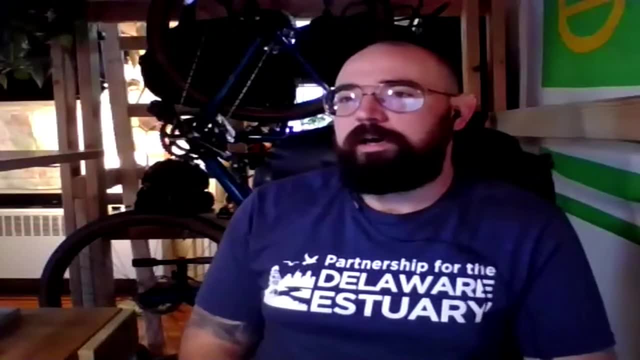 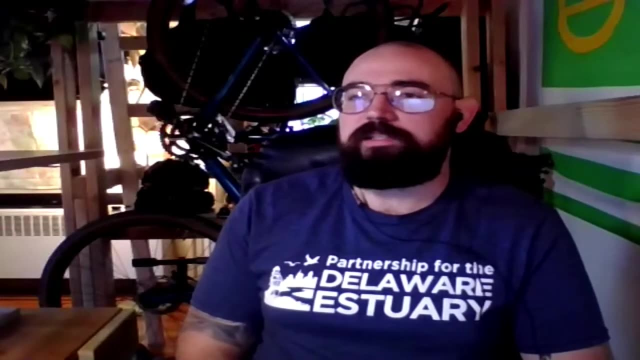 I don't believe we're using any of those sensors. currently. most of our data collection is going out into the field with calipers and YSI or other water quality probe and collecting data manually, and or collecting water samples that we then filter and process manually. so at the moment, at least for freshwater. 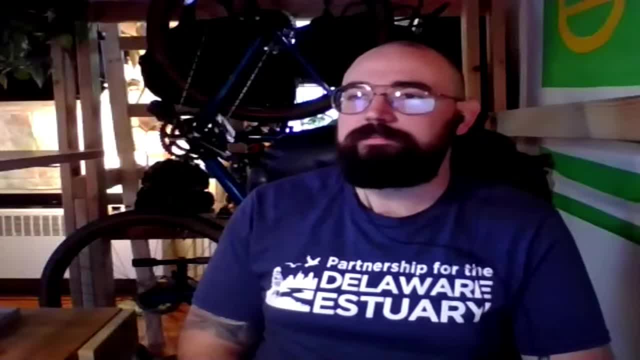 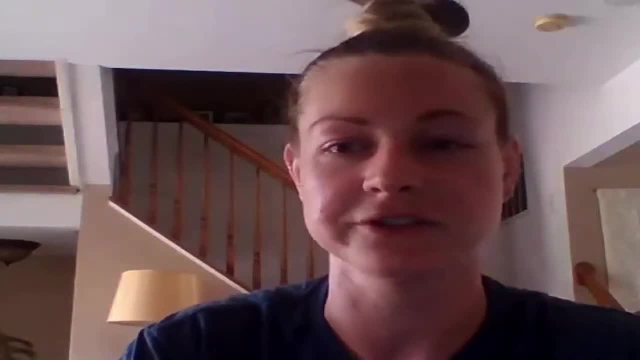 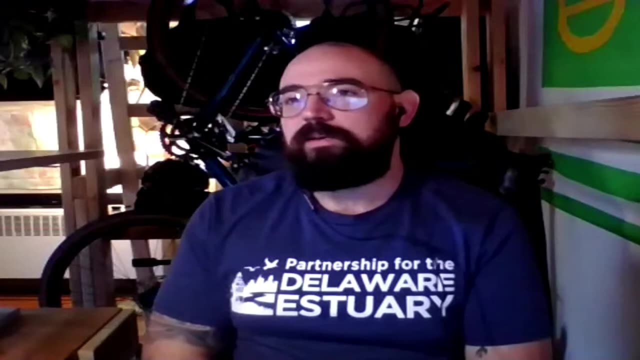 mussels? I'm not aware of any. any of that that we do. all right, great, we'll do just one more. how long do the Glacidia stay attached to the fish gills? that? that also depends on the mussel species, and that's one of the things that we either learn from. 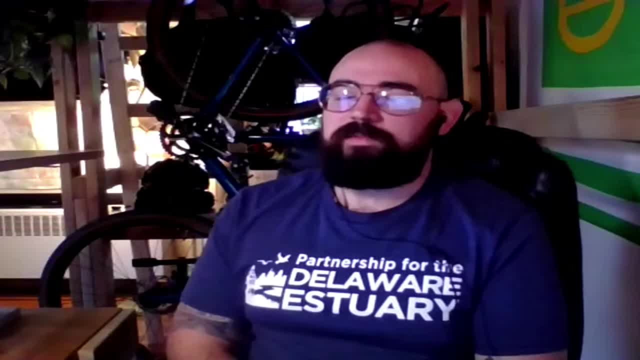 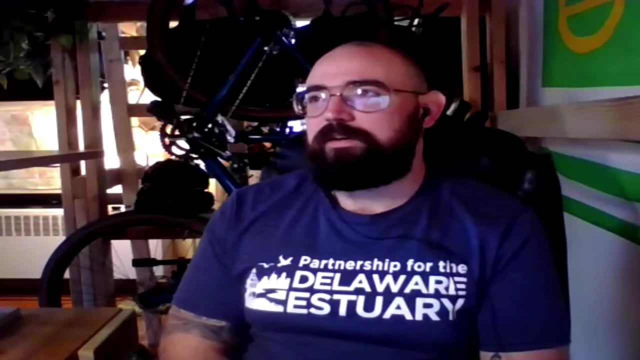 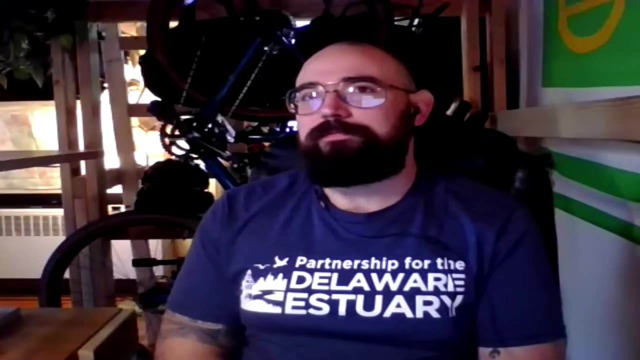 literature, or if there's not good literature on it. that's some of the experimentation and research we can do in the hatchery at the Fairmount waterworks. some species will drop off after ten days, some will stay latched on for three weeks. so that kind of yeah, it depends on. 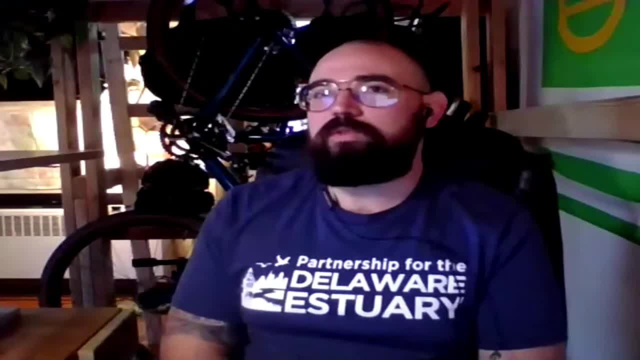 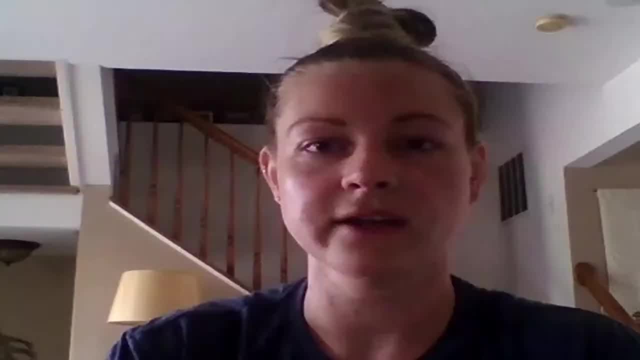 these species of mussel, the species of fish, but generally. between 10 and 30 days is probably a good ballpark estimate. all right, well, great. thanks. so much, Matt, and thank you, Kurt as well. I'm going to just turn it over to Virginia for some wrap-up. great thanks, Emily, and thanks again Kurt and Matt. I'm just 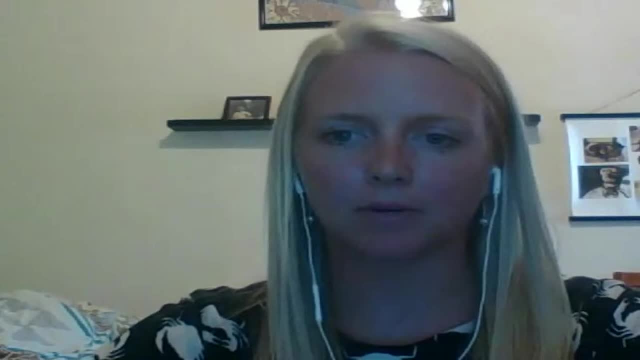 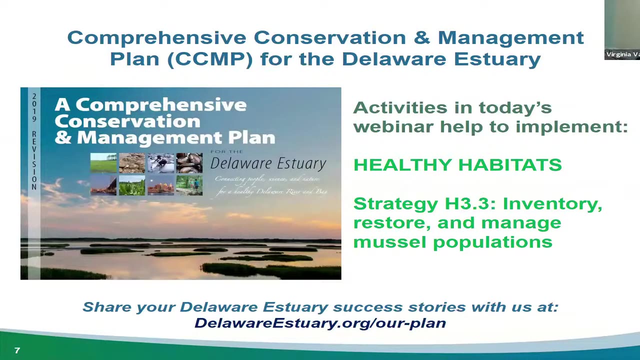 going to share my screen real quick for the wrap-up. so, for folks who aren't familiar with our comprehensive conservation management plan, we wanted to provide a little bit of information for you all today, and so really one of one of the main reasons that we care about this great work with 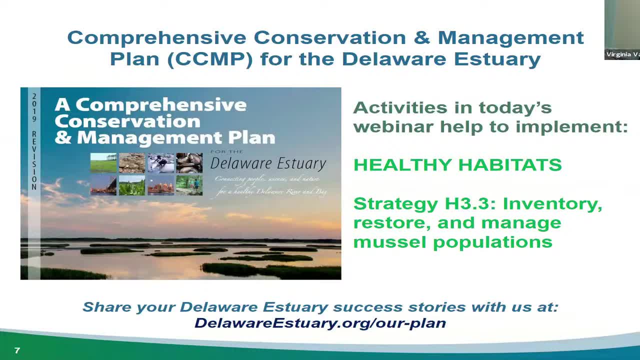 freshwater mussels is because of the efforts to implement key strategies in this CCMP plan for the Delaware estuary, and so the plan was written to guide the efforts of environmental agencies and organizations across the region for watershed improvements, And today's webinar closely relates to CCMP healthy habitat strategy. 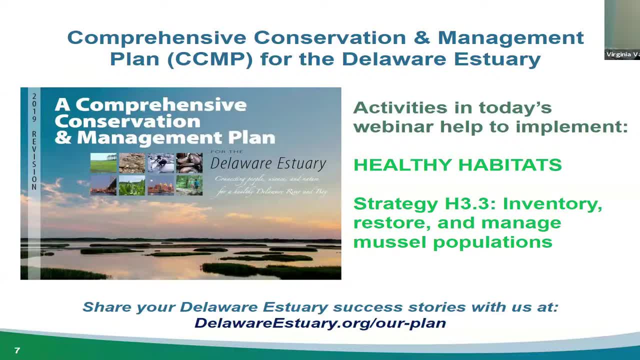 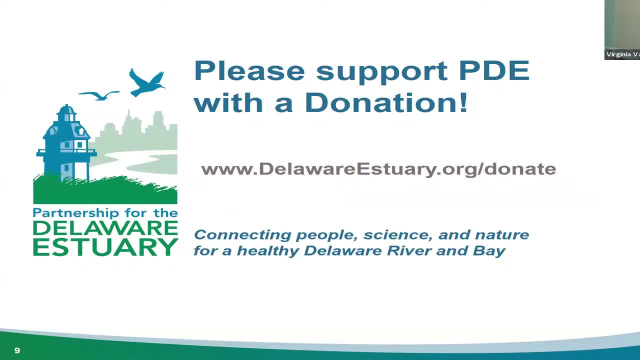 H3.3,, which is to inventory, restore and manage mussel populations, And so thanks again for everyone for attending today's webinar. We hope you found it informative and engaging, and please consider making a donation to PDE to help us achieve our.